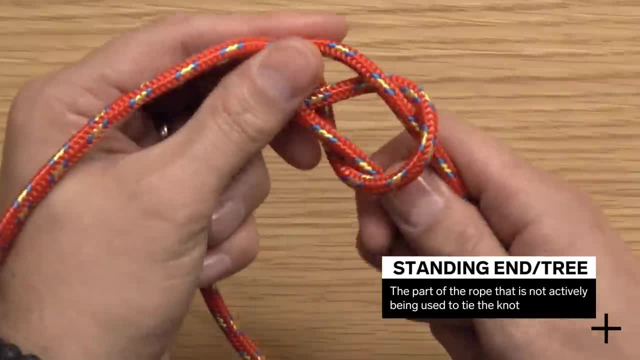 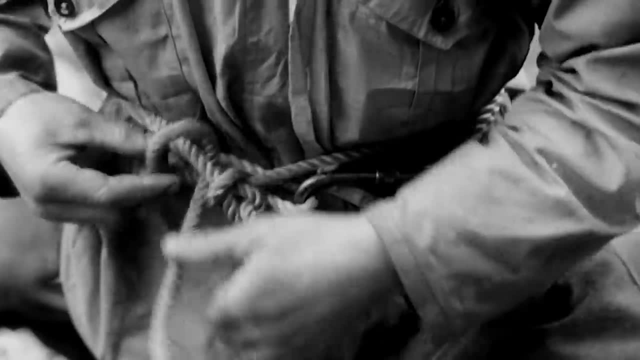 Some people say around the tree And then it cuts right back down that rabbit hole. The bowline is a very useful knot for when you want to create a loop. that's fixed. It doesn't cinch up when the loading end is pulled on. 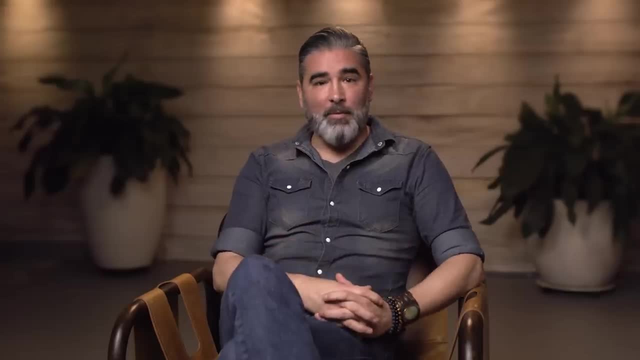 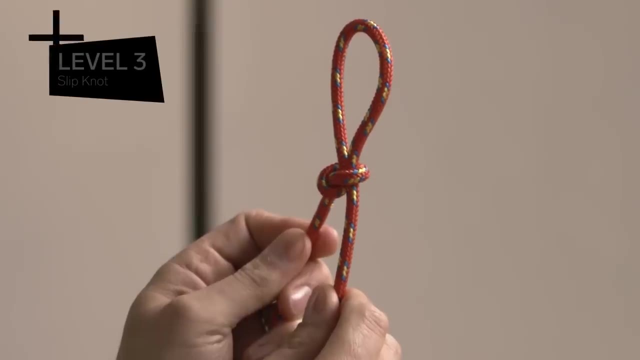 Last thing you want is for you to be in a challenging situation Where you need to be rescued And all of a sudden, as this helicopter or truck tries to yank you out from where you are, you're fundamentally being cut in half. Level three: slip knot. 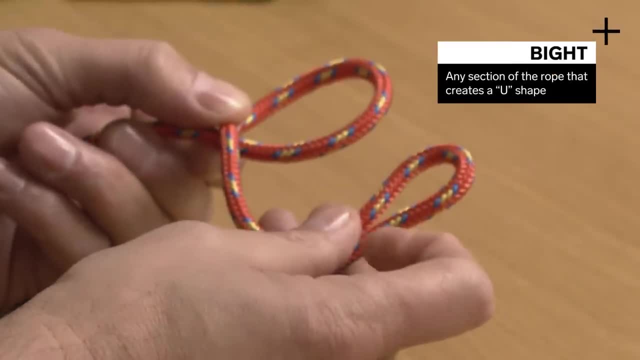 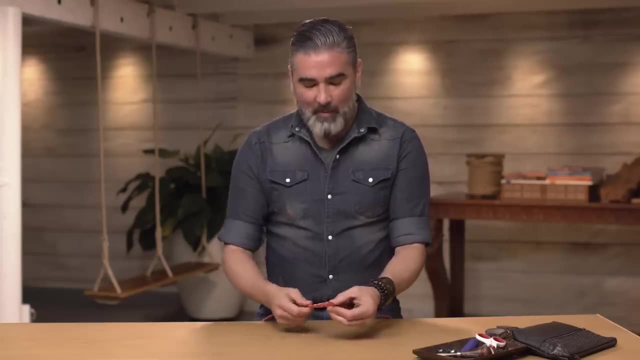 You create a loop, We're going to generate what's called a bite, Just a bend in the rope. The bite is going to tuck through the back of that loop And then we're going to cinch it. What sometimes happens is people have a line on the bottom and they'll try to tuck through the bottom. 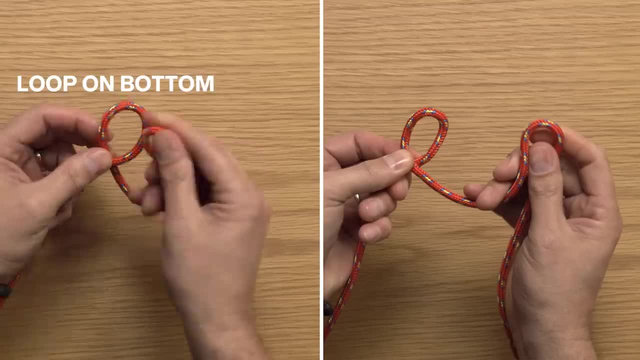 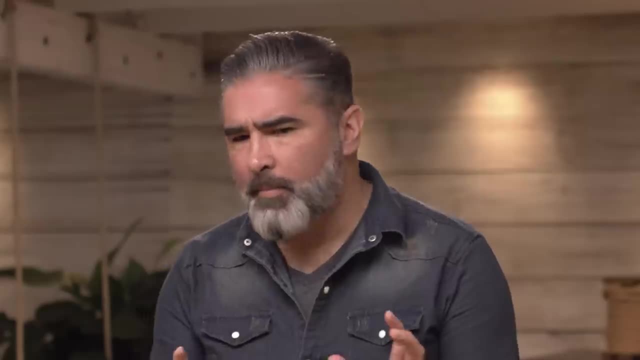 And, as you can see, it kind of just falls apart. If it's on the bottom, tuck it through the top. If the original loop ends on the top, tuck it through the bottom. Now, a lot of times people think a slip knot is kind of an inferior knot because it slides. 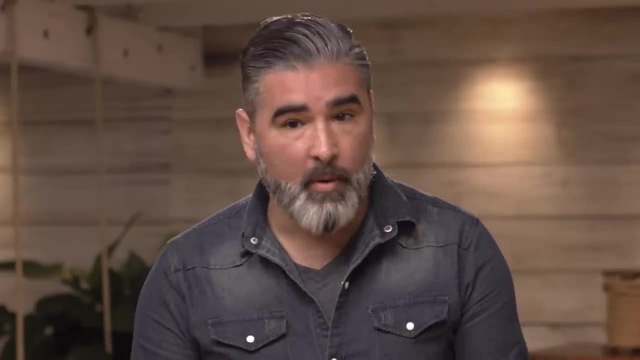 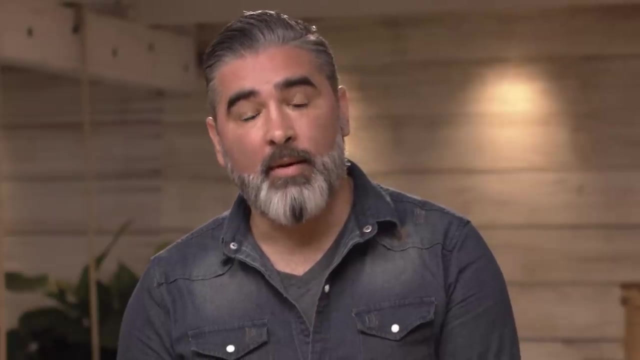 Slip knot, dare I say, is even more useful than a bowline or any other fixed knot. Think about the sweater you might be wearing while you watch this video. That's all basically created with a series of slip knots- The shoes that you might have tied this morning. 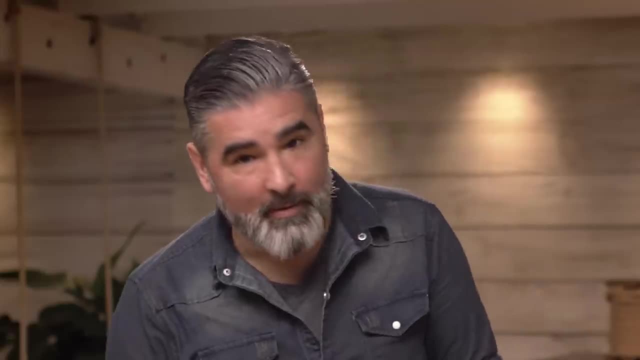 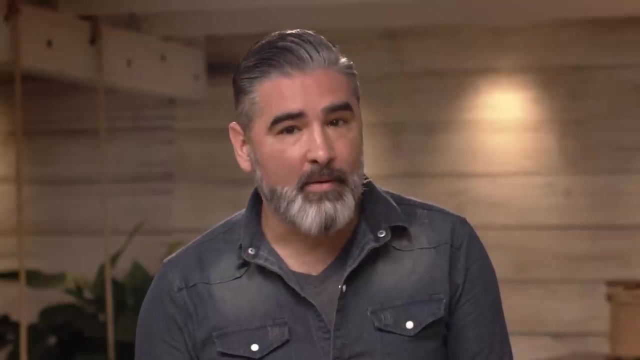 Those are a series of slip knots, So next what we're going to see is how we can take a square knot and make it slightly more elaborate by tying upon itself in a form of a tie that's classically called the Solomon bar, or more recently called a Cobra knot. 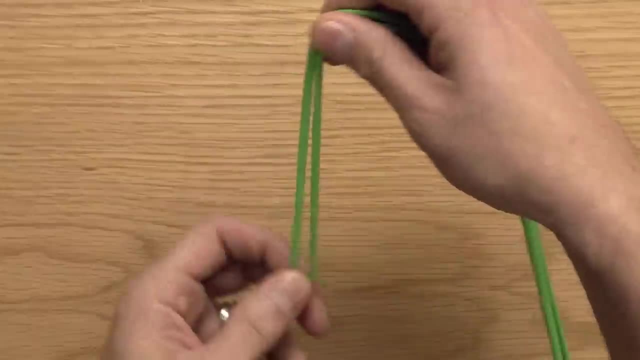 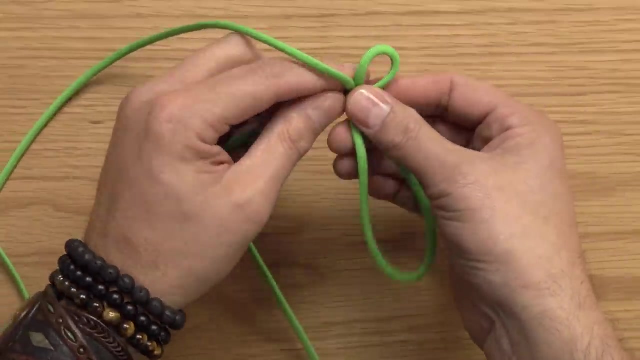 Level four, Solomon bar. So what we're going to do is create a bite. Then we're going to split those cords left and right. Take our right cord. We're going to cross it over the two lines, Then we're going to drop our left cord over that line and then tuck it through the back. 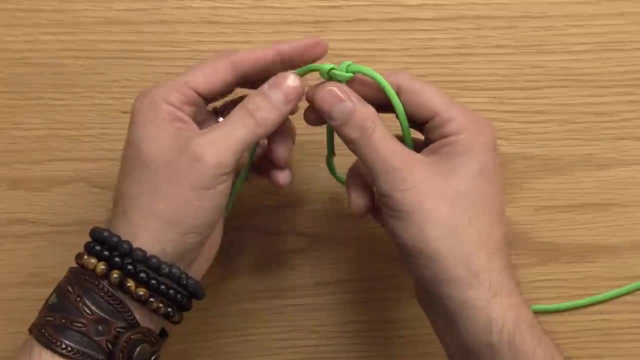 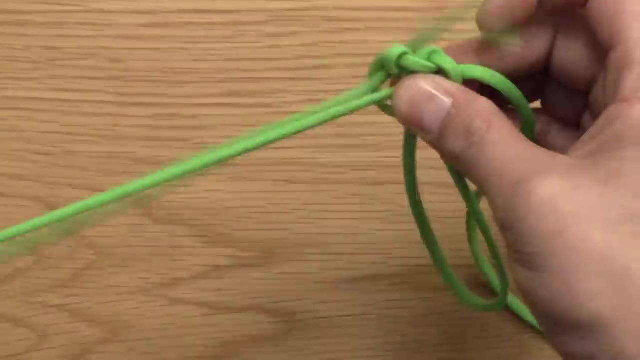 Take up the slack in that to make sure it's nice and firm. Then you're going to take your left line, cross it over, drop the right line over the top, tuck it through the back, Then tighten that up And you have your first overhand knot around the two middle cords. 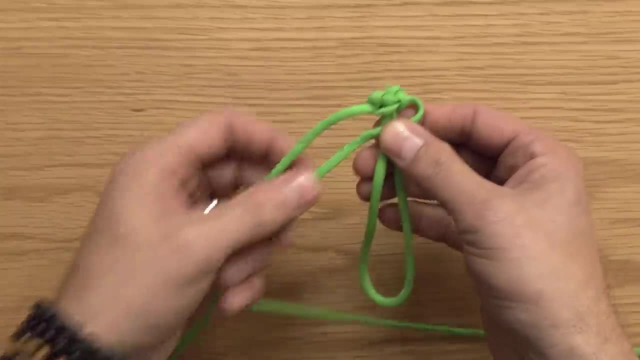 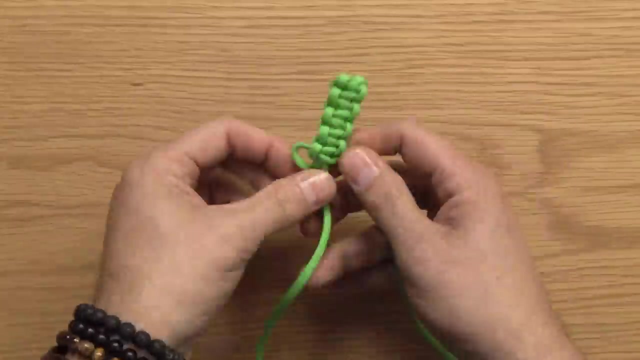 You're going to continue forward, crossing that right cord over the two lines next to it, Dropping the left cord down over it and tucking it through the back. You're going to continue this technique just as before. Solomon bar could be a belt, be a necklace, a bracelet- so many different utilities. 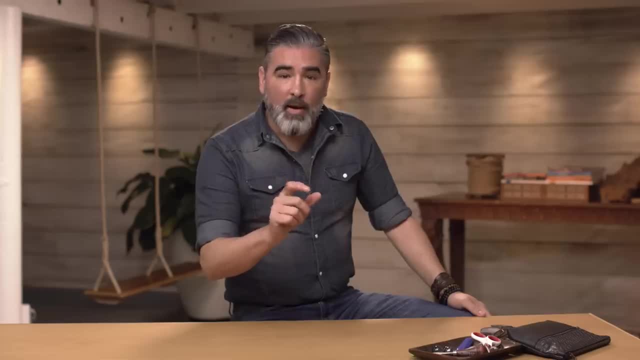 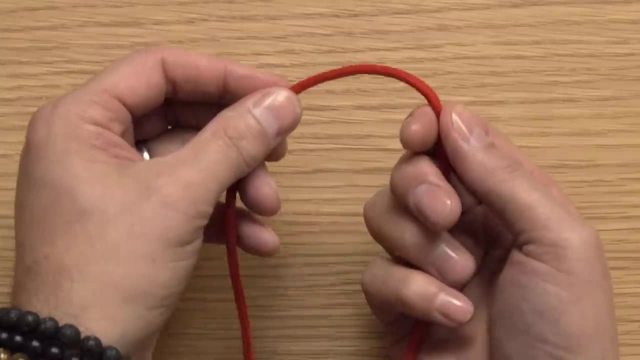 Next up a real clever way of taking a slip knot and turning it into a linear line, Level five: the zipper set. You're going to make a bite, Then you're going to go right over left and then you're going to take. 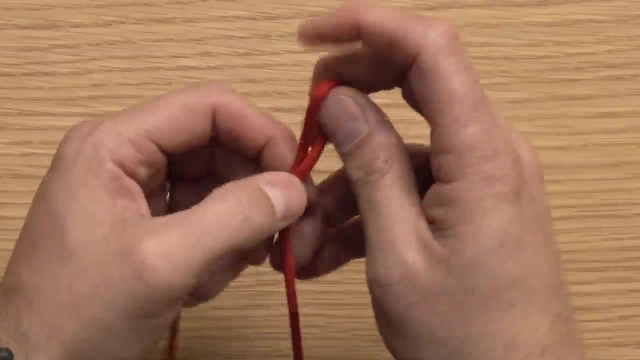 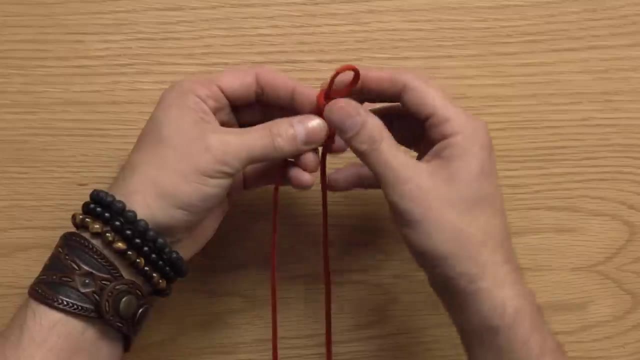 another bite and you're going to tuck it through the loop. Then I'm going to do something kind of slick From here. you're going to take the fixed end and you're going to slide that through the loop, But before I tighten it with the sliding cord on this end, I'm going to pull this out slightly. 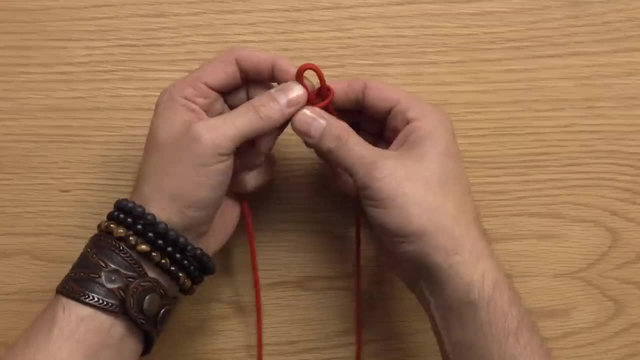 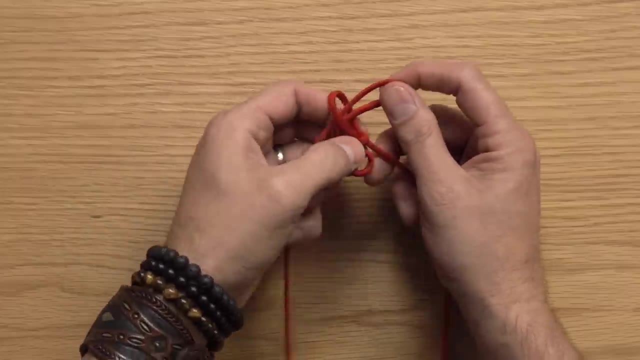 Then I'm going to create another bite that punches through, and I'm going to pull that one taut. So, moving forward, all I got to do is make a bite with the fixed end, slide it through the loop, then cinch it down. 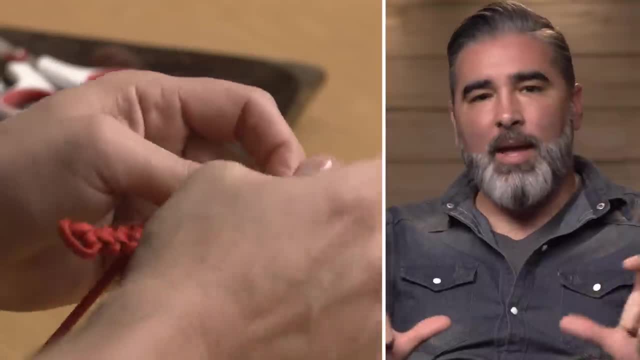 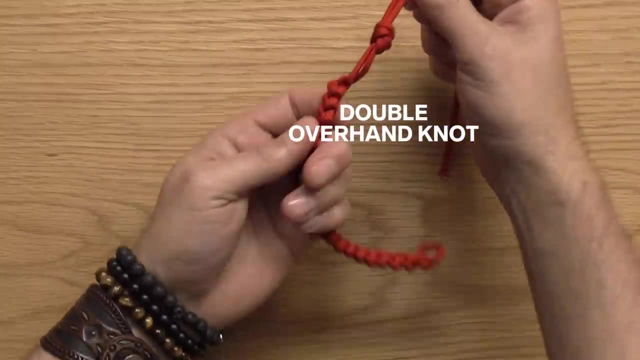 And it creates this really beautiful, almost organic looking leafing structure as you move down, And I'm going to create what's referred to as a double overhand knot. Now, the reason why we call this a zipper set is best explained to you through demonstration. 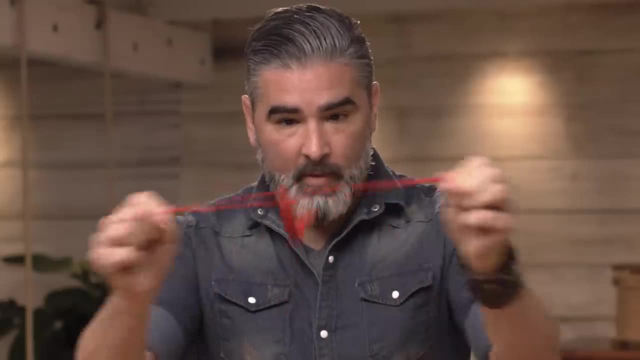 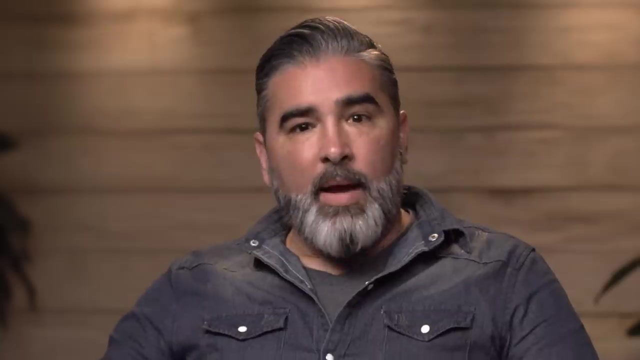 You want to tuck it and then watch what happens. One of the things I really like about knot tying in general is the fact that it's a very simple knot You can do. a few of them go from a usefulness back to the cord with a single pull. 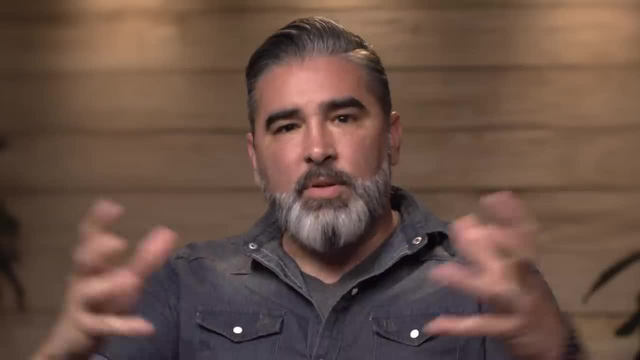 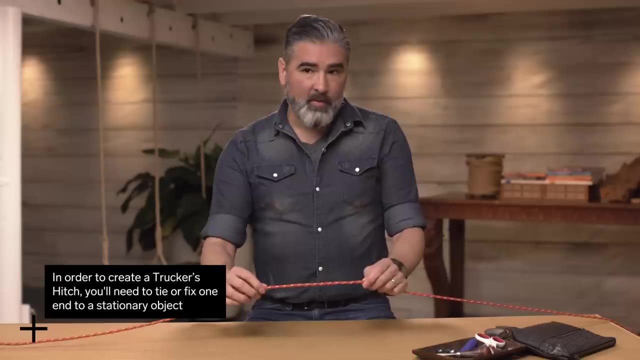 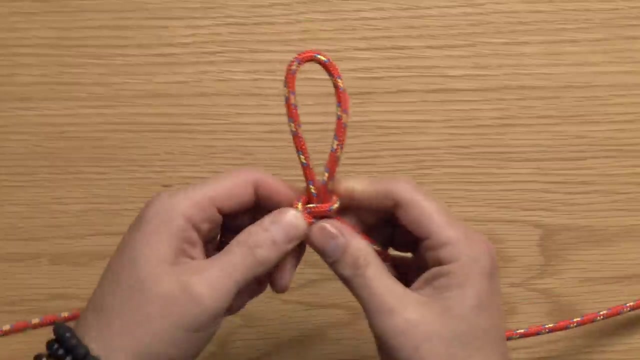 You come to recognize that these tools have so much opportunity to generate so many different things. Level six: the trucker's hitch. You're going to take your line that's going to be fixed off at one point, Then make an overhand loop and you're going to create a slip knot. 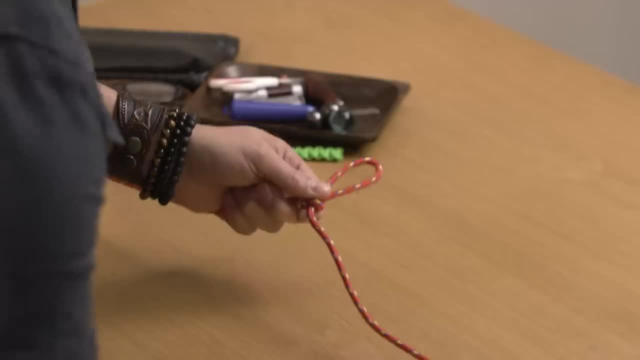 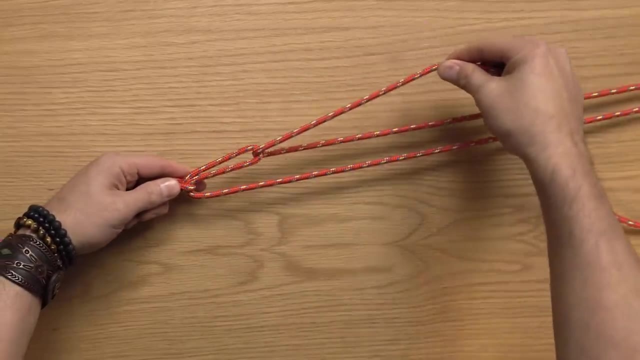 This slip knot is fixed on this end. It slides on this end, but that's okay, Take your other end and you're going to fish it through that loop. This, right here, becomes where the mechanical advantage is achieved. Now, once I get the sufficient amount of tension, 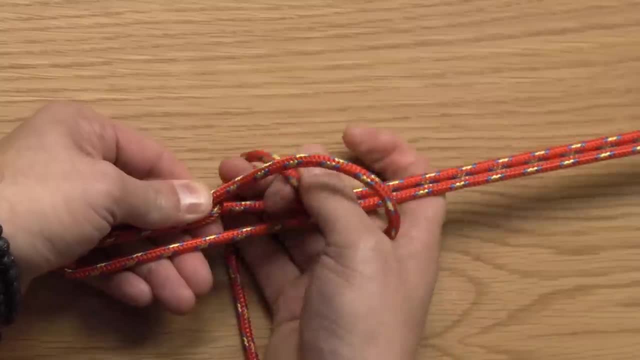 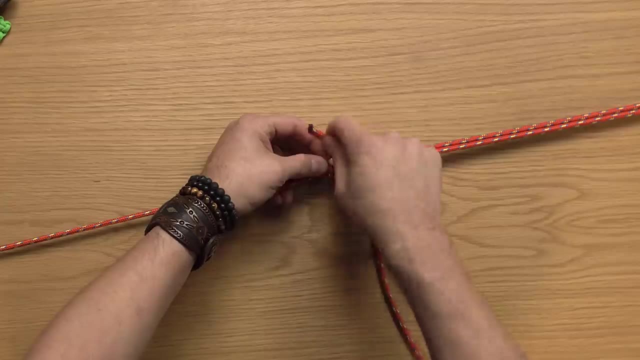 all I have to do is just take my thumb and then create what's called a half hitch. Now that one half hitch will lock this trucker's hitch in place, But just to be sure, I'm going to do the same thing in reverse. 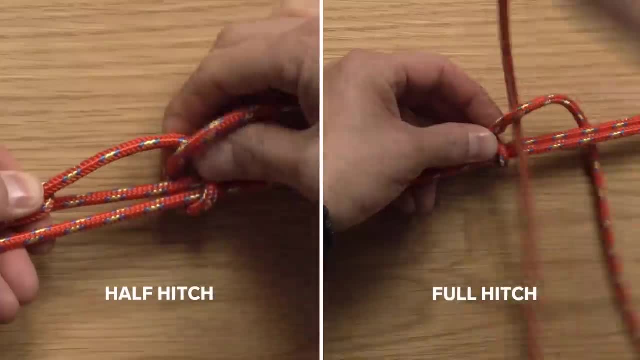 What that's going to create is a full hitch. So I went from a half hitch to a full hitch, with a line in series creating a trucker's hitch. So I went from a half hitch to a full hitch, with a line in series creating a trucker's hitch. 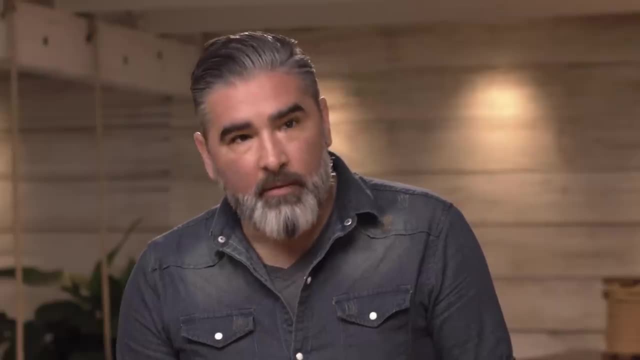 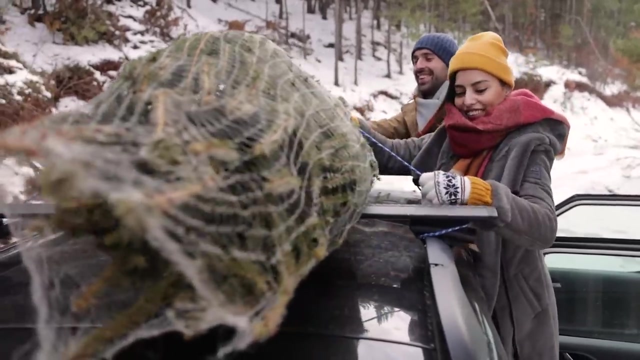 Now a trucker's hitch is achieving a mechanical advantage by creating a series of pulley points without the pulleys. So if you're strapping something down, a trucker's hitch is really the way to go. Going into the next level, we're increasing complexity by adding two ropes together. 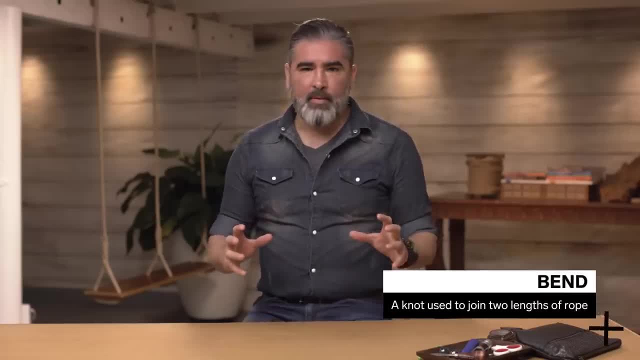 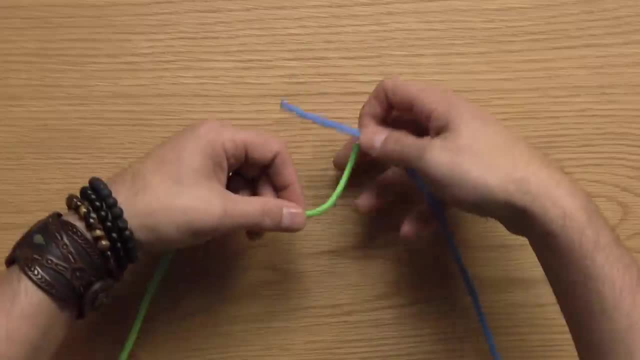 Level seven: bends. A bend is fundamentally when you want to connect two pieces of line or rope. Starting off, I'm going to show you the fisherman's knot. You're going to take one of the lines and place it in front of the other line, in opposite directions. 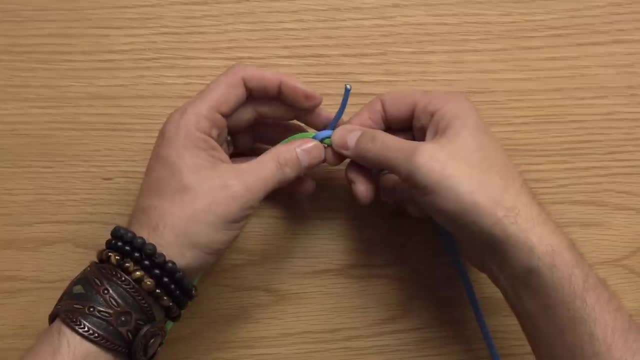 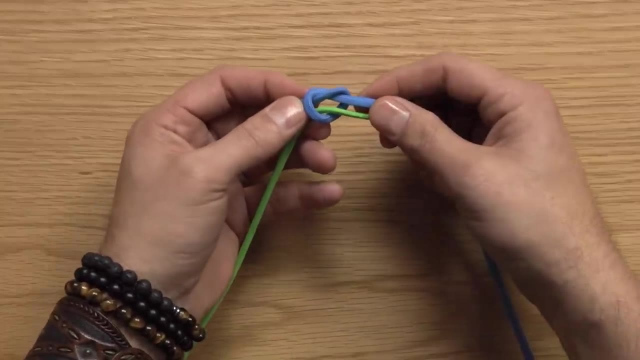 Go over the line next to it and then itself- And this is very important because you don't want to come up between the two- And then through the loop that you've created. Look, familiar, It's an overhand knot. You're going to cinch that tight. 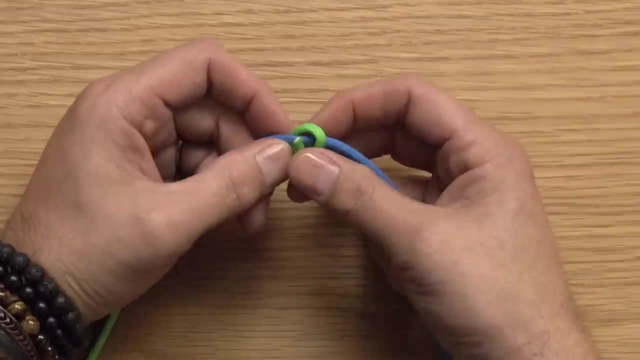 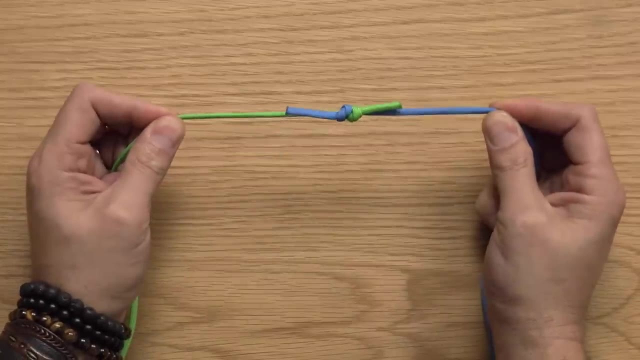 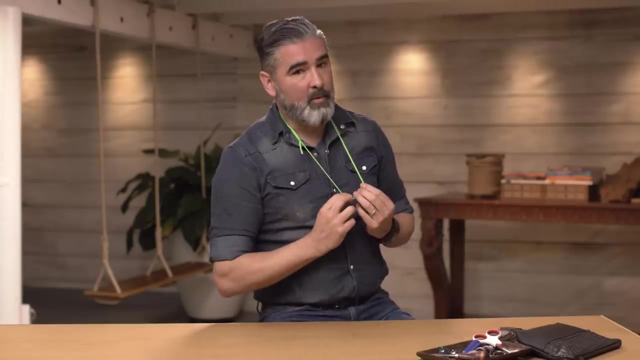 Then you're going to look at your other side. You're going to do the exact same thing in reverse. Once you create these two overhand knots in opposite directions, you pull the load, they slide into each other. So this is a great way of adjusting the length of the cord or necklace around your neck. 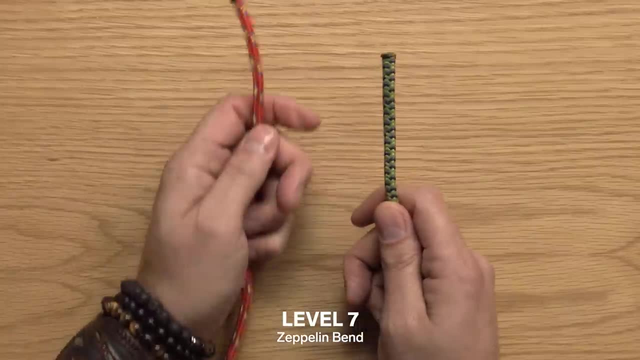 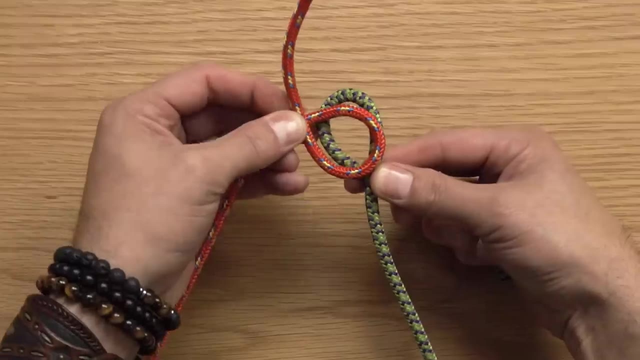 In some cases, you might find yourself needing to connect two pieces of line that aren't the same size. We're going to make a six with our green rope. We're going to make a nine. Take the six and put it on top of the nine. 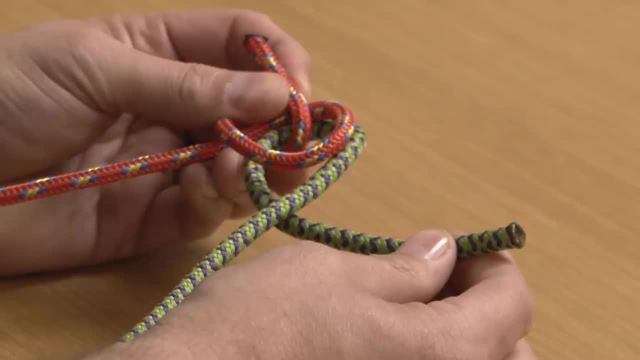 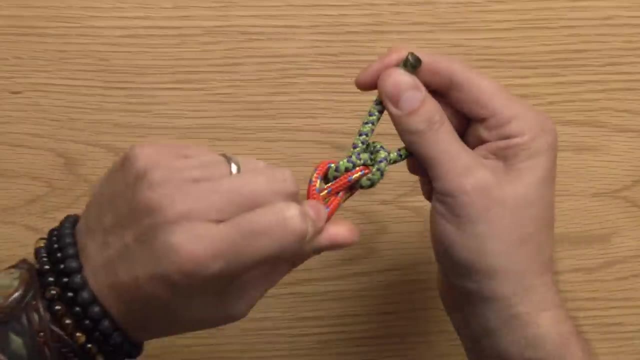 You're going to go down and then up through the middle, And then here it's going to go up and down through the middle of that loop. Once you've generated this configuration, you're going to pull on your standing ends to create a zeppelin bend. 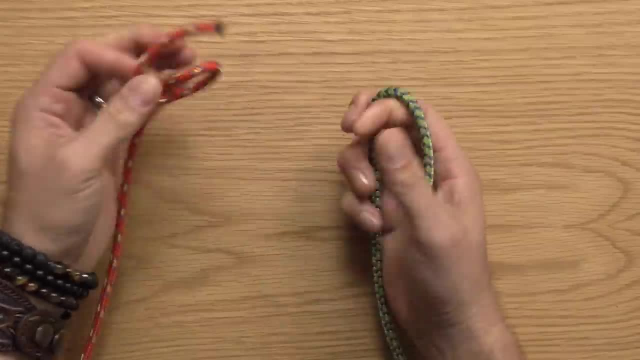 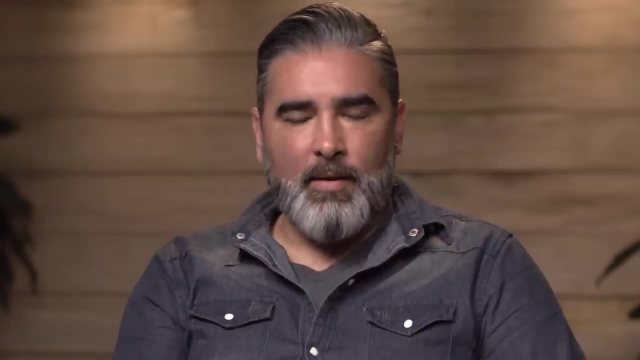 And then, when you're done, you can separate the rope ends with ease. When I'm tying a practical knot like a bowline and a zeppelin bend, I find the utility really inviting, But there's nothing that really draws me in from a cultural perspective. 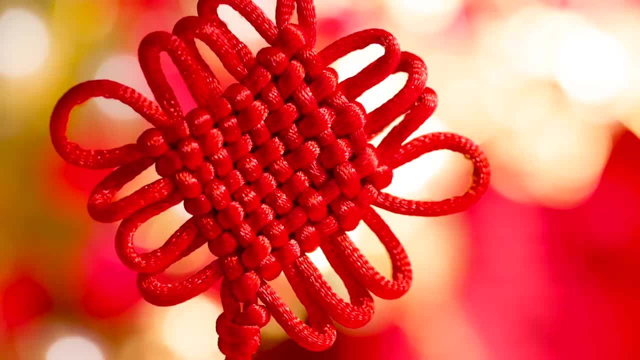 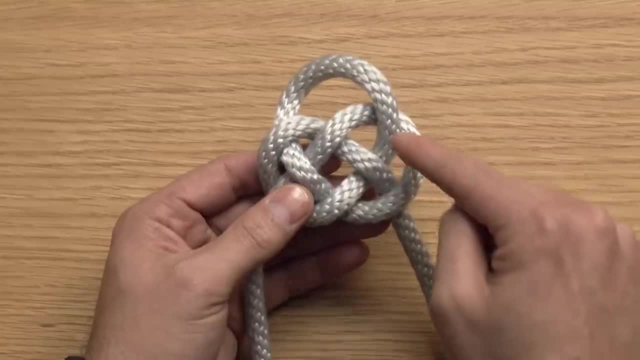 When we talk about more decorative knots or pieces that have spiritual or sacred significance, those draw my attention. They're like acquaintances that I miss and in some cases want to celebrate. Level eight: the double coin- There's so many elaborate decorative pieces. 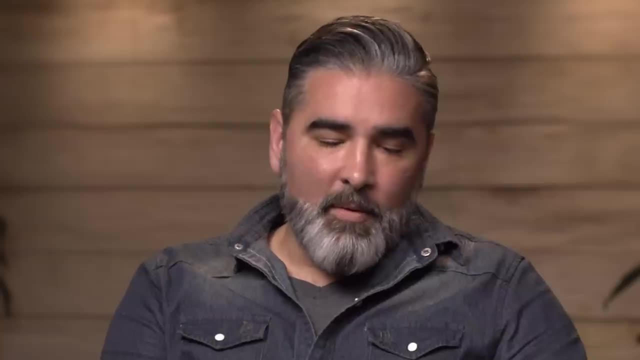 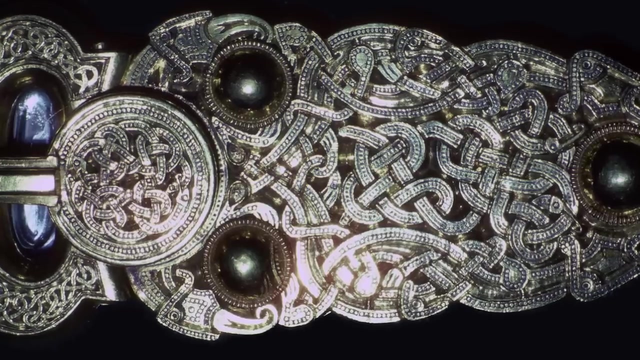 that can be created from the double coin knot. It's also the base of many traditional knots from Mesoamerican cultures, Germanic culture, Eastern Asian cultures and the British Isles. I'm going to start at the middle of my rope. I'm going to make a P with the left side. 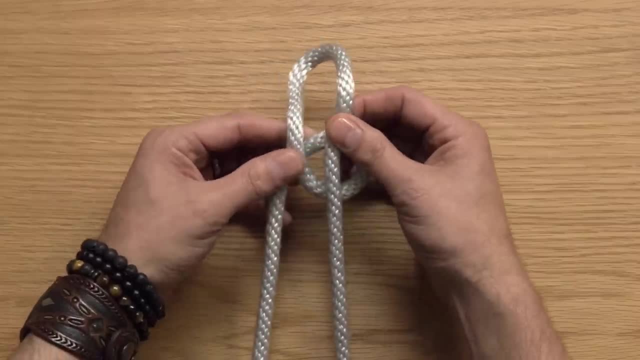 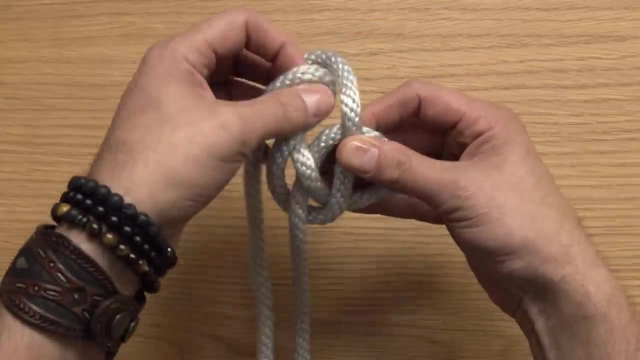 Then what I'm going to do is I'm going to take the right cord and I'm going to cross that eye just like a finger in front of your eye. Then this end is going to go under point one, then over point two. 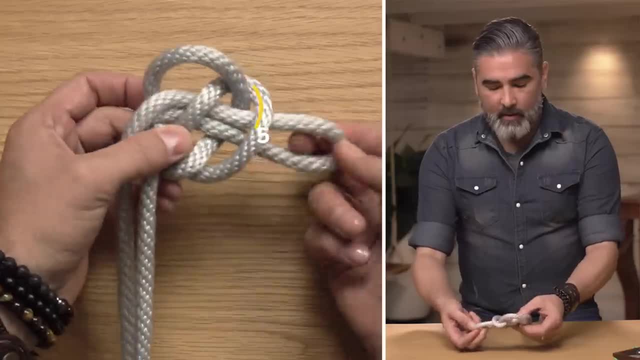 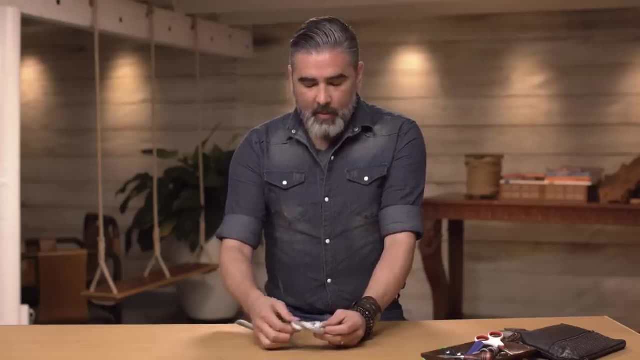 under point three over itself and then under that last point. on the bottom, You can see that diamond pattern in the middle. But I want to point out that I didn't fish for the end of my rope, I just took a bite and threw that bite through. 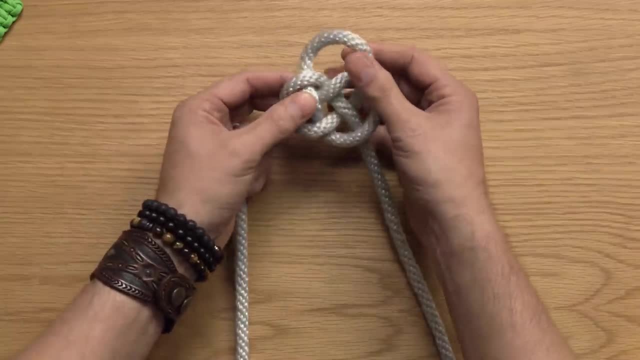 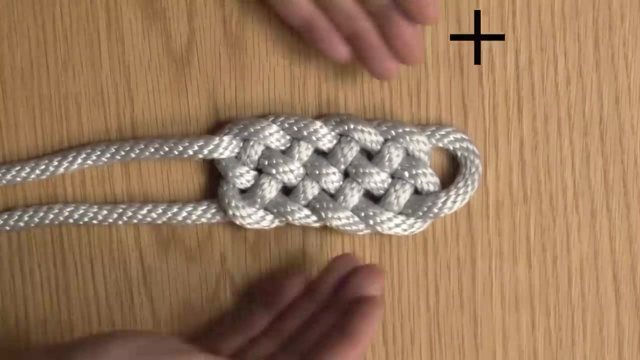 then I pulled it out. It's a little trick of the trade. For our next level, we're going to take the double coin knot and we're going to expand it longitudinally, as if two coins overlapping wasn't enough. Level nine: the prosperity knot. 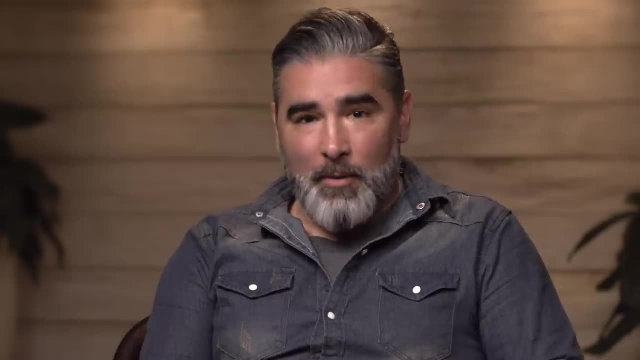 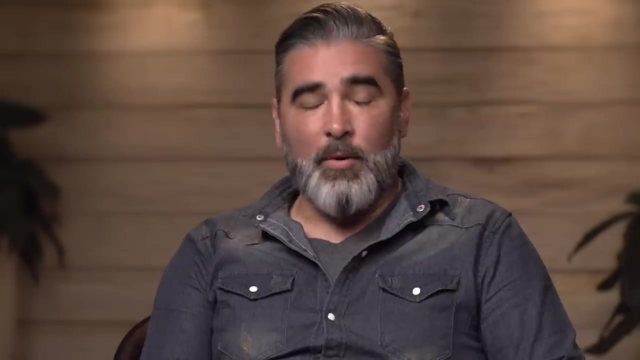 The prosperity knot is kind of a clever knot. It's a historical knot in the sense that it's been around for quite a long time, but its structure is very similar to a fusion knot. So in a way it is kind of a historical fusion knot. 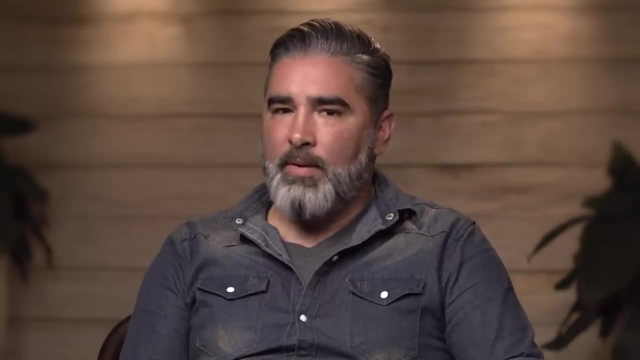 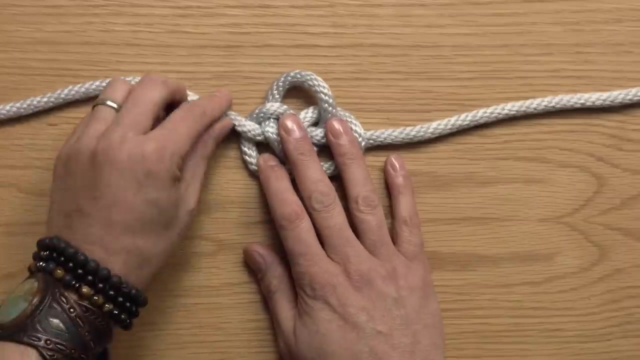 Now, as far as its utility is concerned, that's really up to someone's creativity To transition a double coin knot into a prosperity knot. you take your running ends and you're going to pull those out to the side. Then you're going to take up a little bit of slack. 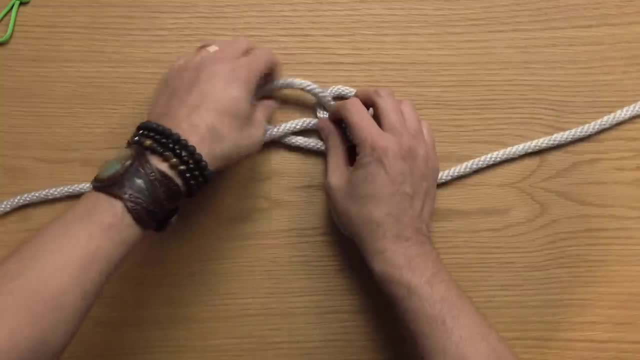 I'm going to pull that down and I'm going to take up a little bit of slack on this side. What that'll generate is kind of like these wings on the bottom. Then what you're going to do is you're going to take 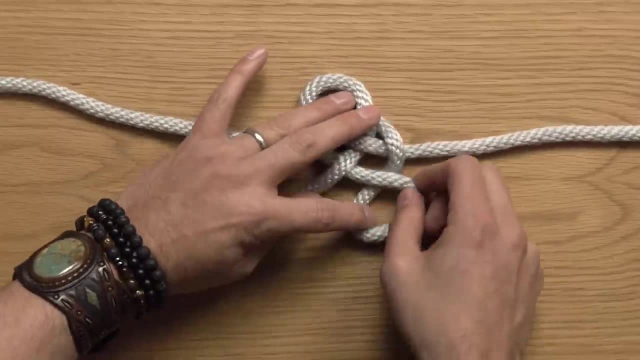 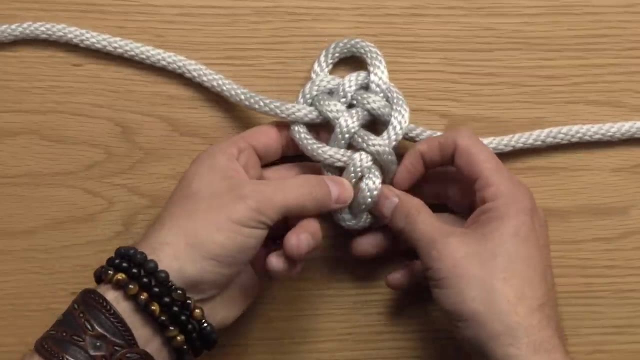 this bite that's down here and you're going to go left over right, I'm going to go over to your left side and repeat the same thing. So then you're going to take this loop and it's going to go underneath the left edge of the loop next to it. 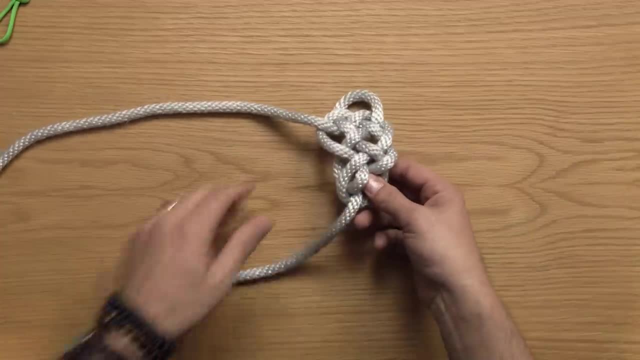 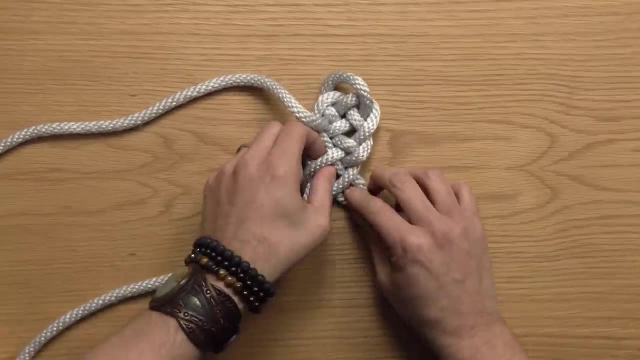 This rope is going to travel over the eye of that loop below And then you're going to fish this over that rope end and through the bottom of the end next to it, And it's going to create this kind of configuration. Now all we have to do is take our left side of our rope. 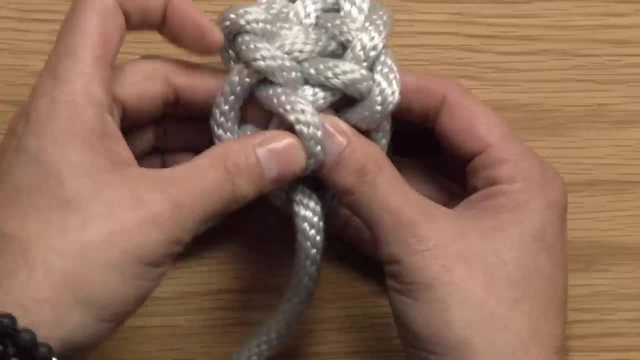 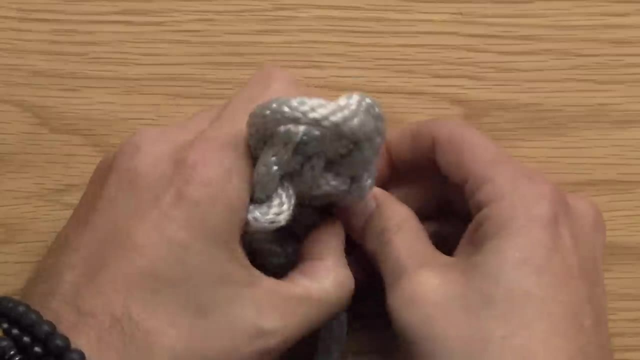 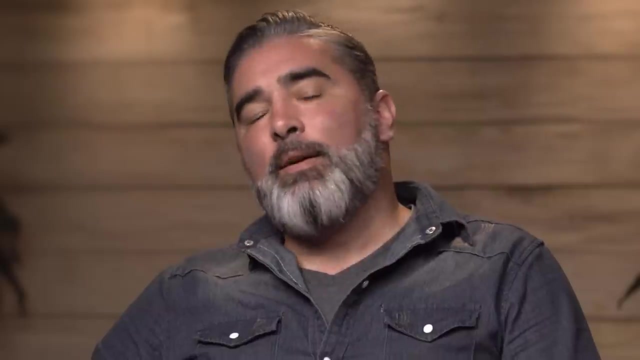 We're going to go under point one, over point two, under point three, over point four and under point five. I'm going to pull that through to generate what is referred to as the prosperity knot. Is it a decorative knot? Yes, 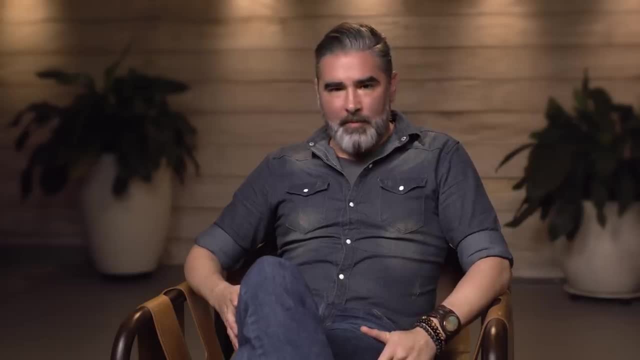 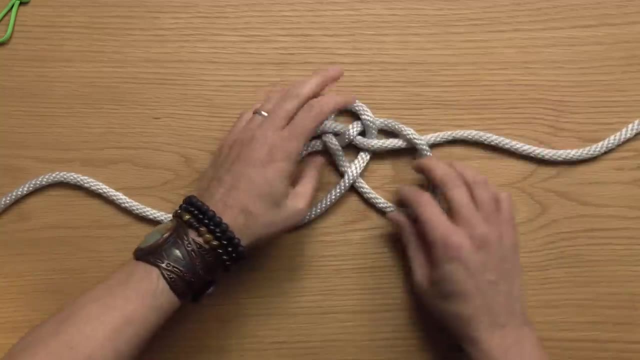 Can it be used for utilitarian purposes? Absolutely. Once you understand the fundamentals of the weave, you can actually reorientate it into a variety of configurations. While we're on the subject of decorative knots that are sacred to various cultures, I thought it would be really interesting to show 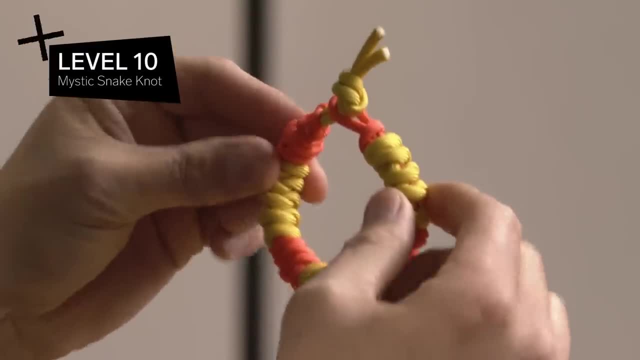 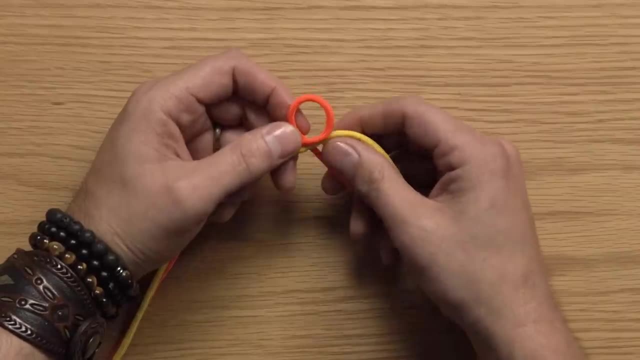 a knot that's referred to as a snake knot Level 10, the mystic snake knot. You take your top cord here and you're going to make a loop. Then you're going to take your bottom cord and line it up with that top line of the loop. 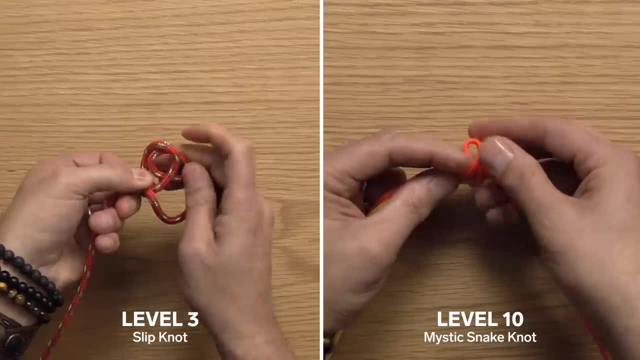 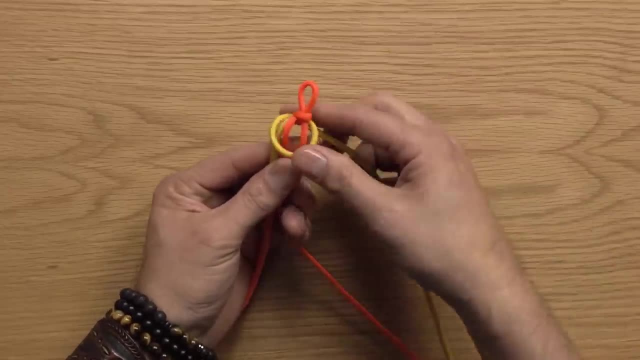 And then this right here is going to punch through and generate- you guessed it- a slip knot. You're going to take your right cord and you're going to curve it to the left all the way around the piece. Then this cord here is going to come around the back. 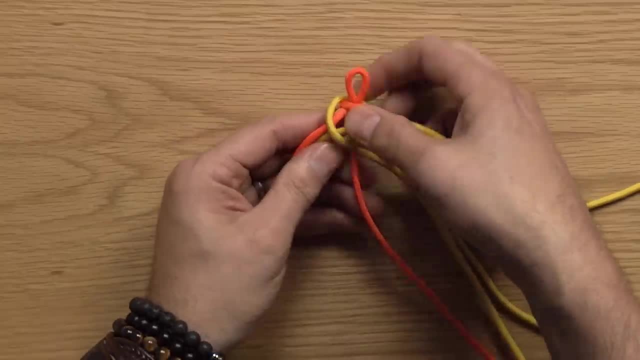 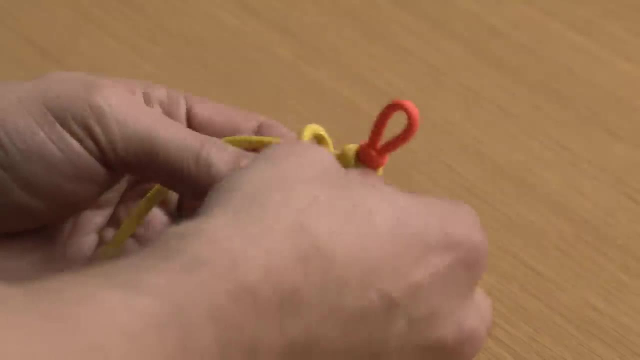 and then down the left side. Then you're going to take up the slack, tightening it nice and firmly, Then you're going to continue forward just like that. This particular piece, a lot of the technique, is in the adjusting, making sure each knot as you stack it on top of each other. 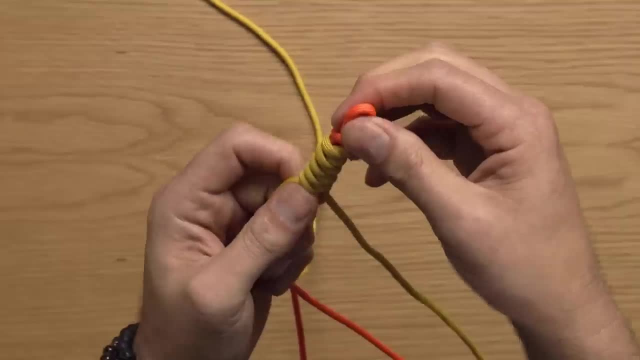 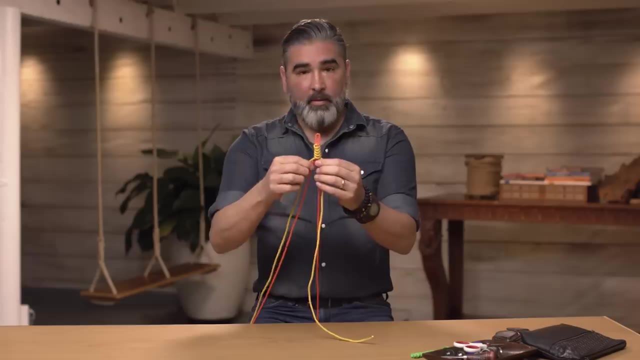 is adjusted proportionally to the one below it. If one knot is loose and the other knot is tight, you'll notice a difference. I'm going to show you how you can transition from this color, this yellow, to the orange beneath it. 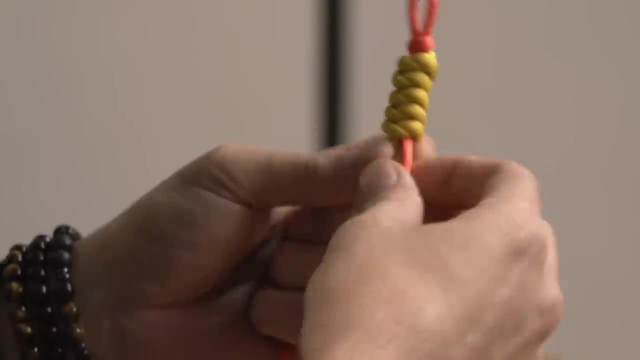 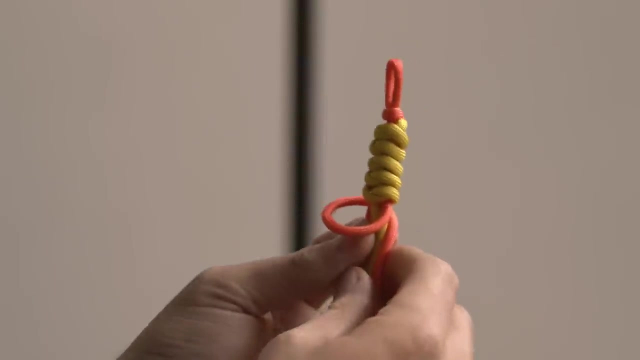 The way you do that is, you're going to take the yellow pieces to the middle and the orange pieces to the outside And you're going to do the exact same technique, except now you've just changed the color. This is one of the first times I'm illustrating. 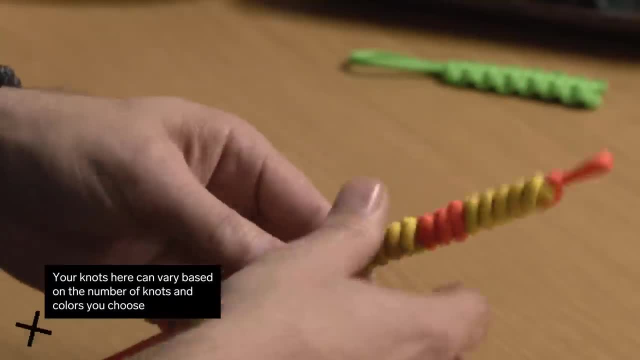 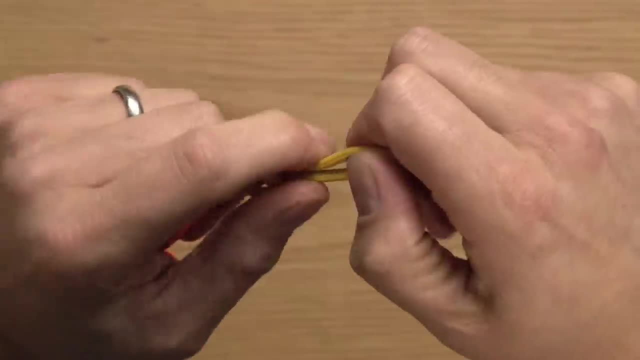 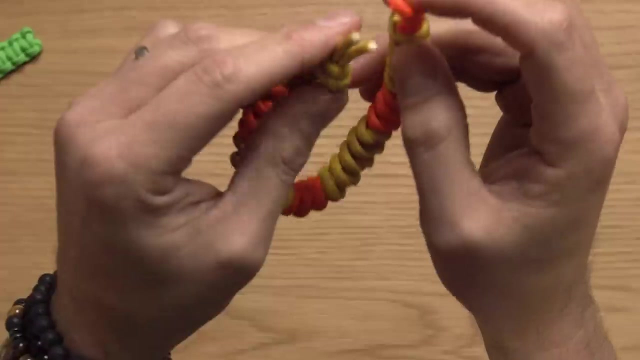 a knot that you could spin your own creative input into The details, the nuances. it's your choice, your creative vision. I finish it with just a square knot: snip it there, torch glass, those ends, And then you have this. 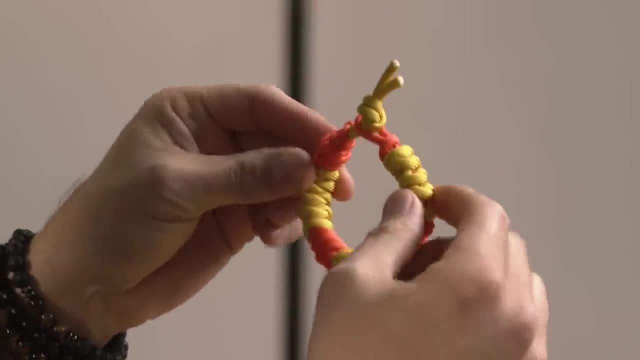 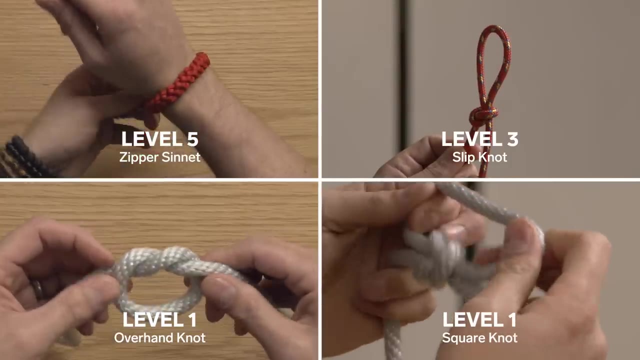 tucks through and there you have it: a mystic snake knot made into a bracelet. So now we're going to move into the advanced knots, where we're going to take sinets and slip knots and overhands and square knots and we're going to mix them all together. 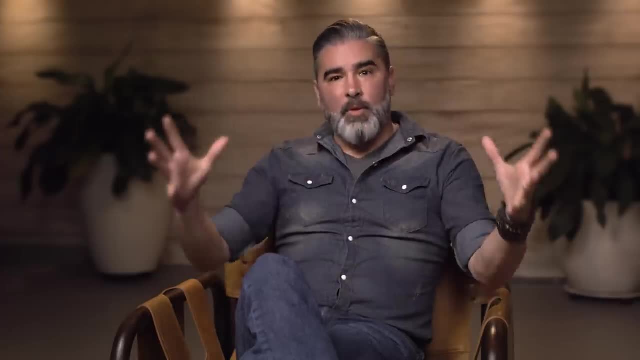 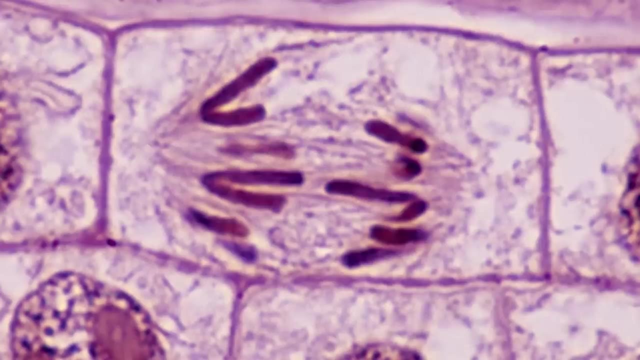 to make something more elaborate, more detailed and more complex. Level 11, the spindle fiber bar- The name comes from- during cellular division, there's something called spindle fibers. My background is biology, and so when I was looking at the way these 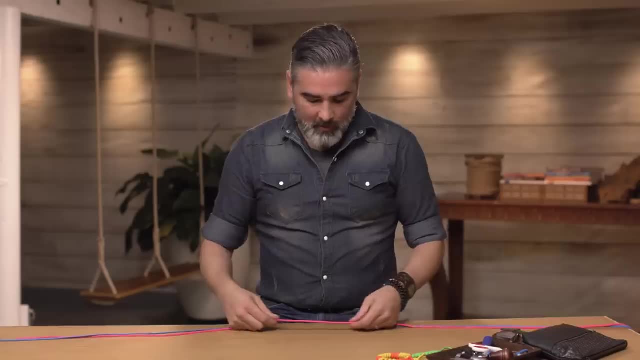 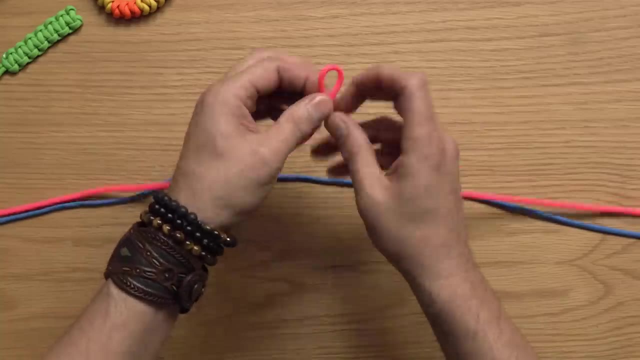 interlocking hitches looked. it looked a lot like spindle fibers to me. First, you're going to take two lengths of cord. My blue length is about six feet and this one's about three feet. I'm going to bend our short line. 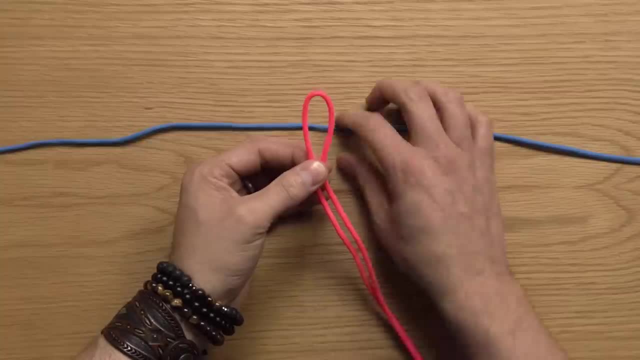 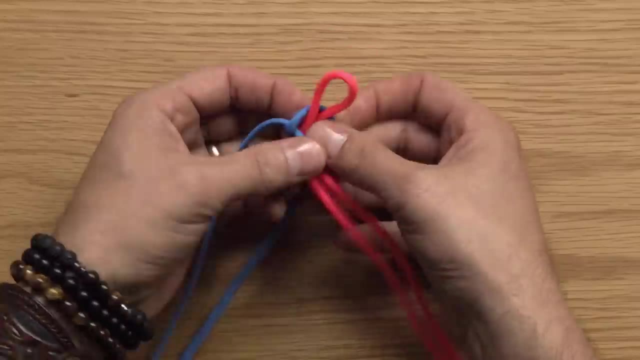 creating a bite at the middle of the cord, Then I'm going to take our long line, put it behind, I'm going to cross over, drop this one down and then I'm going to tuck that through the back And this, fundamentally, is just an overhand knot. 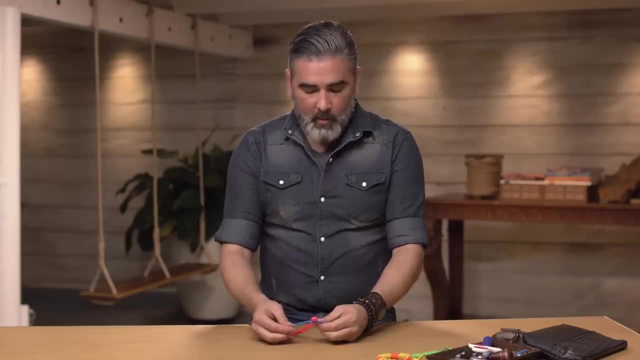 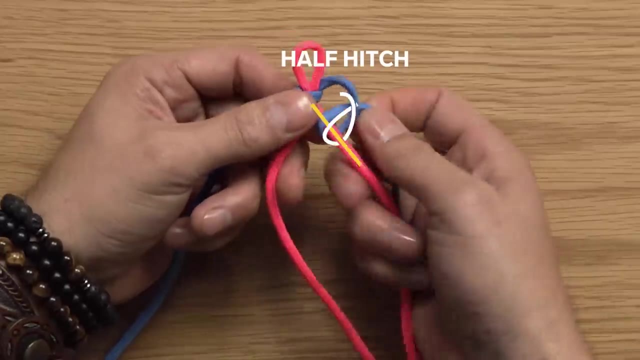 wrapped around two parallel lines. Then I'm going to take our cord on the right side, tuck it underneath the cord adjacent to it and through the loop created, And that is just a half hitch. Now notice, I don't tighten that up yet. 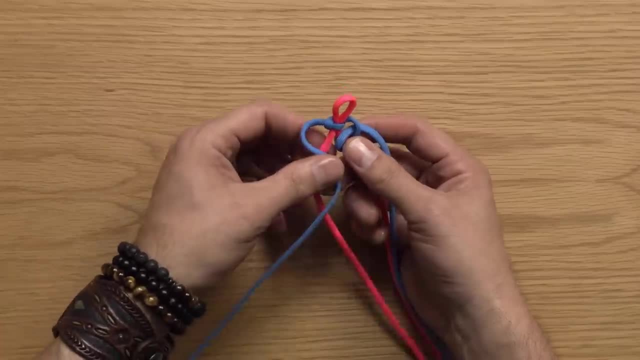 We're going to leave that loose for now. Then what I'm going to do is I'm going to take the line on the left, I'm going to go over the line next to it, I'm going to fish for the end. 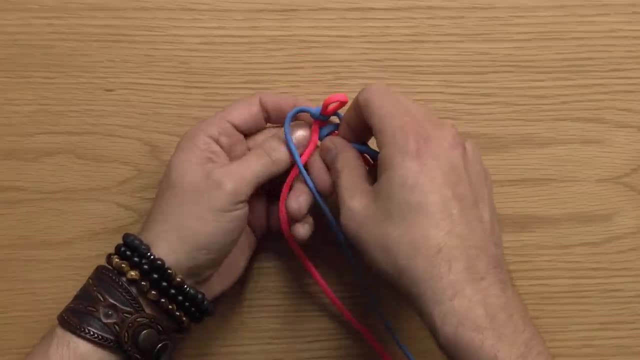 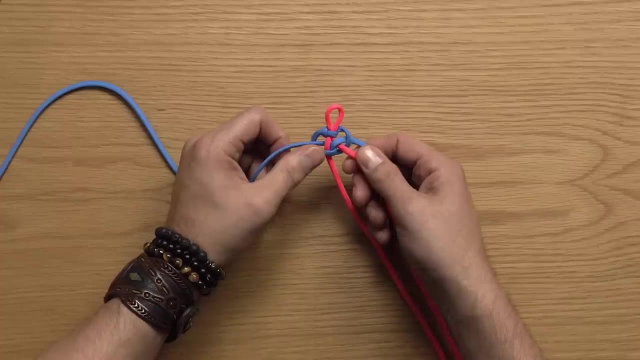 and I'm going to go down the loop associated with that half hitch on the right and I'm going to cut up. So I've created another half hitch, but this one goes over behind and then up through and this one goes under over. 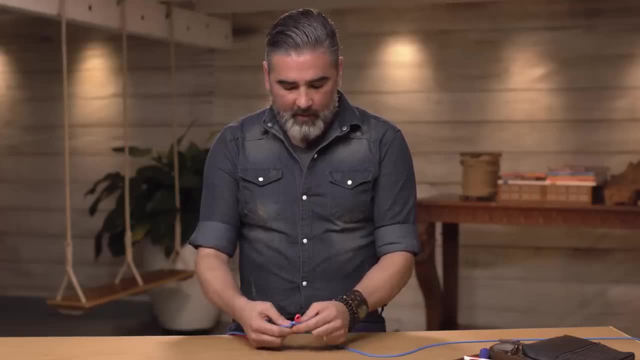 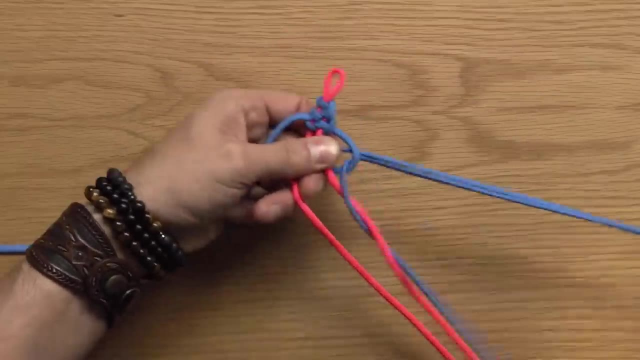 and then down through. So this demonstrates a little subtlety about half hitches. Just because they're half hitches doesn't mean you can't do them two different ways. This same technique is repeated all the way down, And so once again. 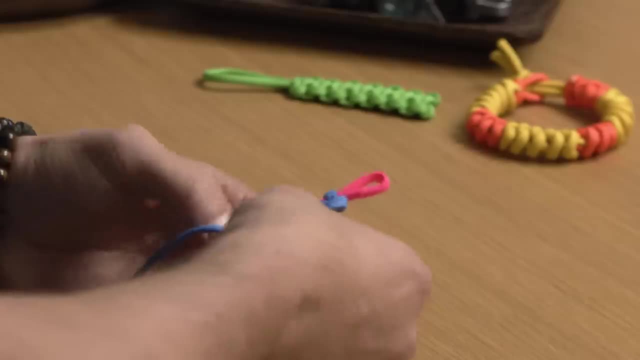 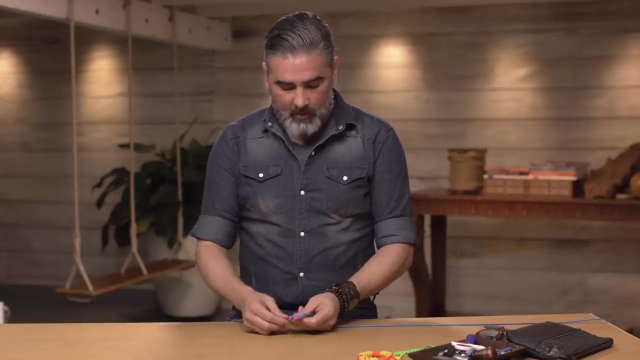 the complexity isn't in the actual technique, but as the pattern extends itself it starts to create something synergistic. so the hole is bigger than the parts. Just like before, we're going to snip off those ends and then we're going to cut up the loop associated with that half hitch. 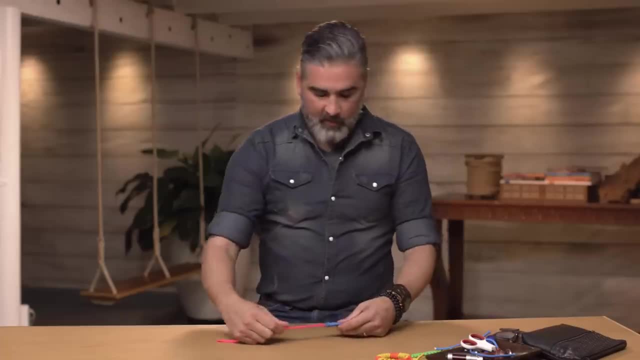 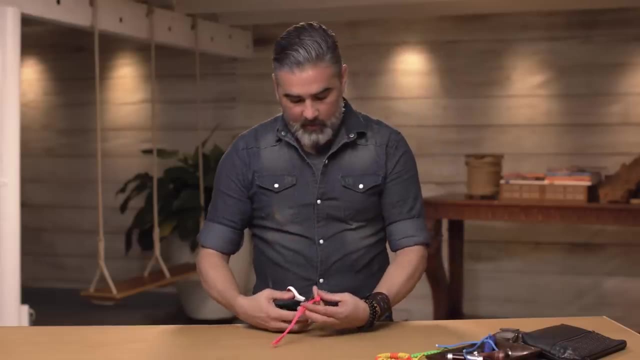 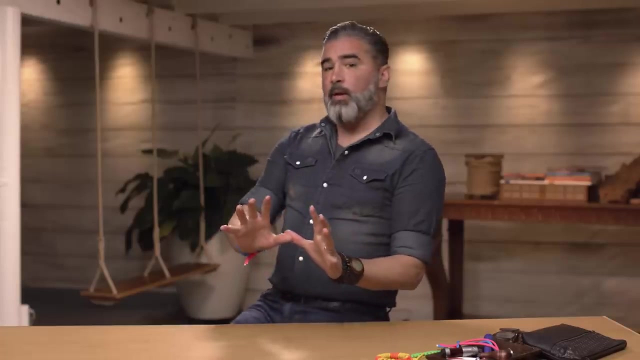 Take our ends, take our torch and with the center strands just going to do a double overhand knot. Just as a side note, I always like to leave a little bit of tether at the end For our next piece. what I plan to show you is a little bit more advanced. 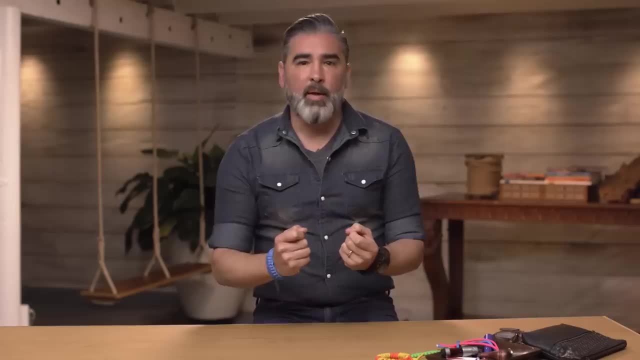 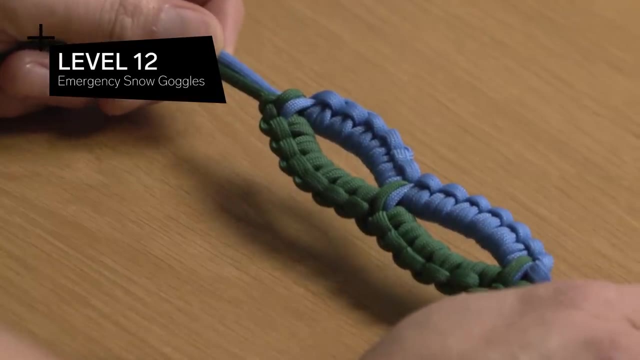 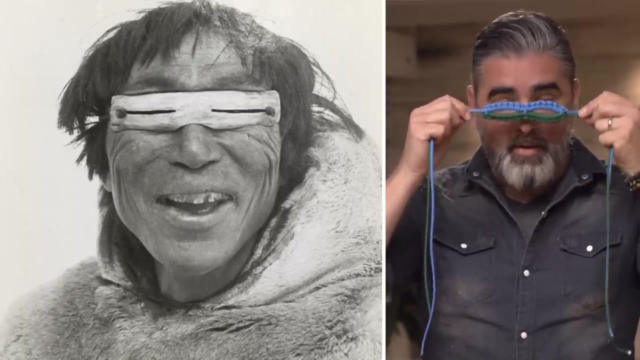 than the spindle fiber bar, but it's going to take those fundamental methods, in this case a half hitch that may one day save your eyes. Level 12, emergency snow goggles. You're going to take your emergency snow goggles to reduce the amount of UV light that enters the eyes. 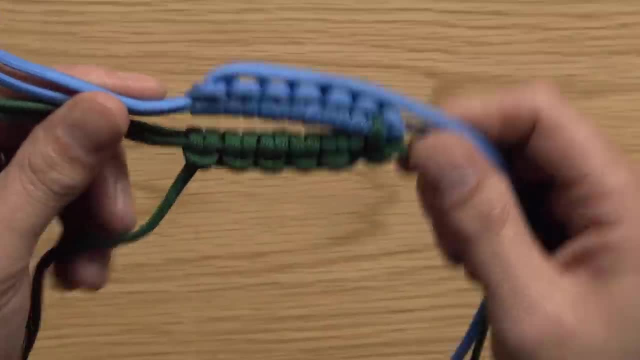 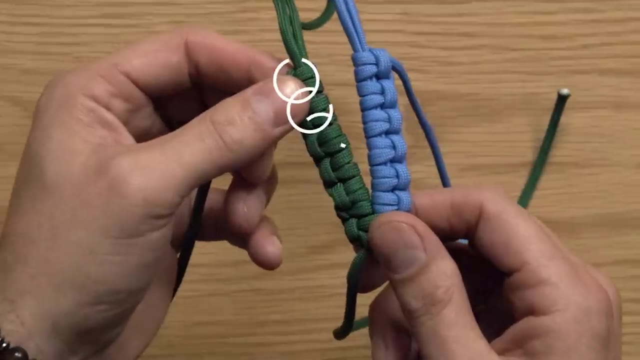 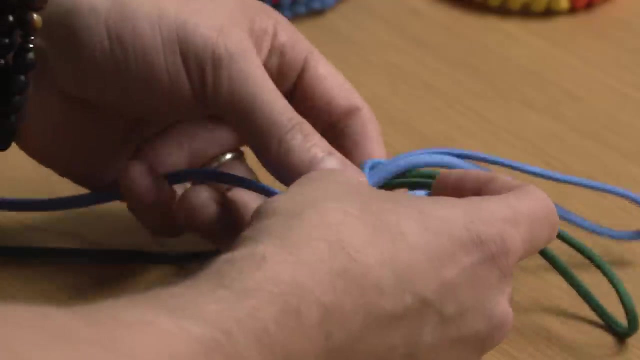 and subsequently saving you from going snow blind. Start off with half hitches stabilizing the base and then full hitches along a right-hand line and along the left-hand line. You're going to take your right cord. it's going to tuck underneath the two vertical lines. 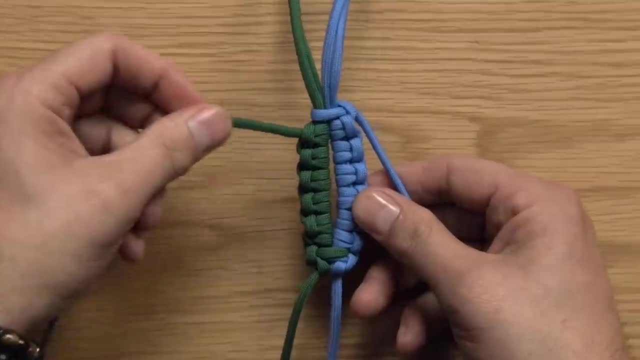 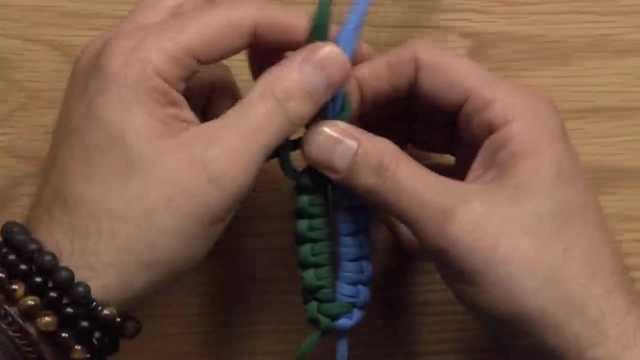 then over and through the loop created. Then take the left cord and you're going to tuck it underneath, and then over and through the loop created. This is the middle point where the bridge of the nose will go, Then moving forward from here. 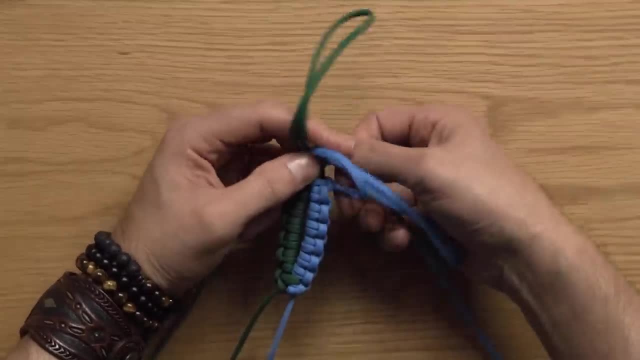 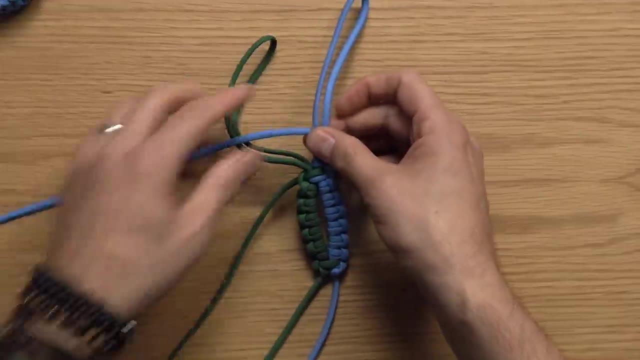 take this line and you're going to go over the two vertical lines above it and through the loop. Then you're going to go under the two vertical lines above it and through the loop, Now doing over and then under with a half hitch. 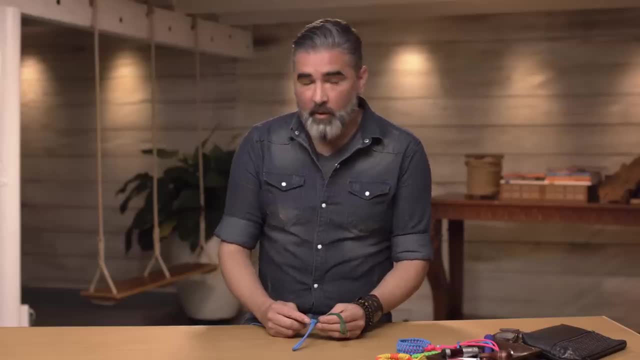 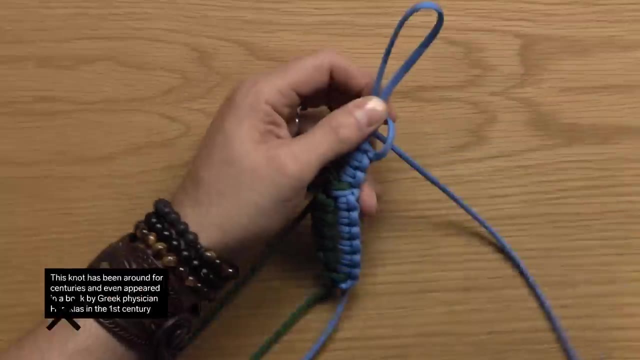 is going to generate a full cow hitch. It's also called a lark's head. You're going to continue this pattern, moving up the strands above until, in this case, you generate six stacked full hitches. As a side note, 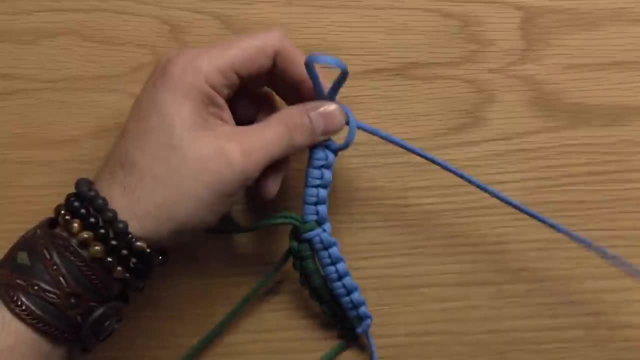 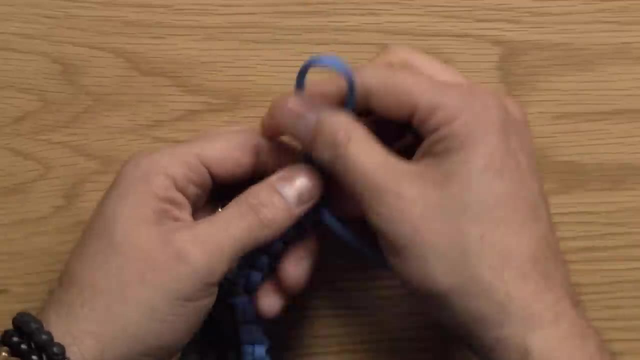 many people mostly encounter a cow hitch or a lark's head off the middle of a rope, but you can also generate it, as shown, with a single strand in one direction. You just have to know how the knot is oriented. Same thing on the other side. 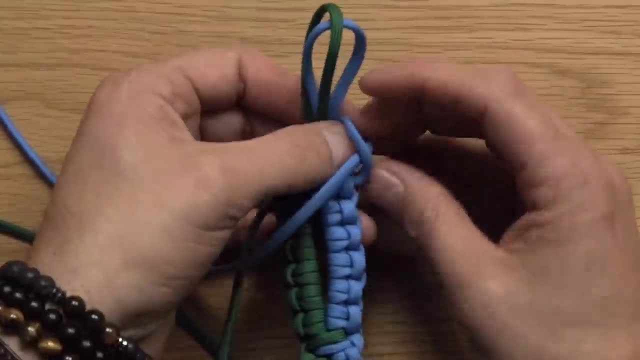 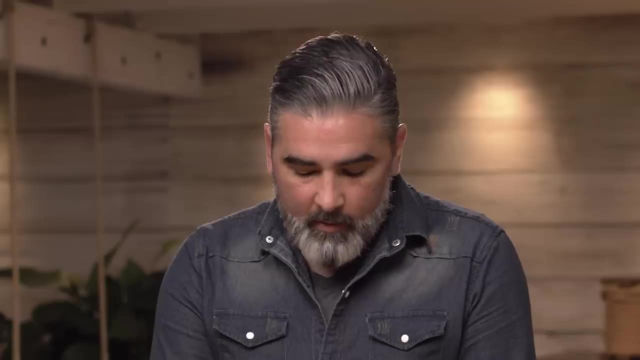 and then, to finish it, you're going to go underneath, over the top and through the loop created, creating a half hitch. I know you're thinking this, so I'm going to go ahead and say it: Yes, they can double as superhero masks. 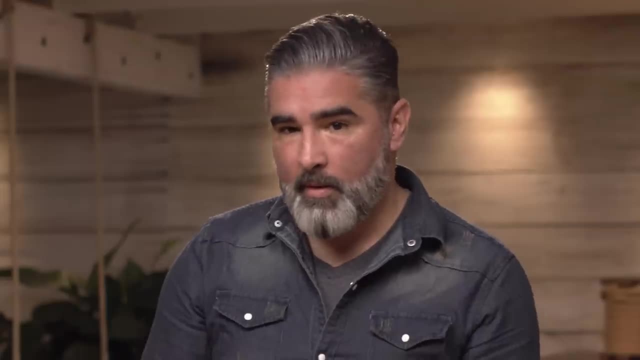 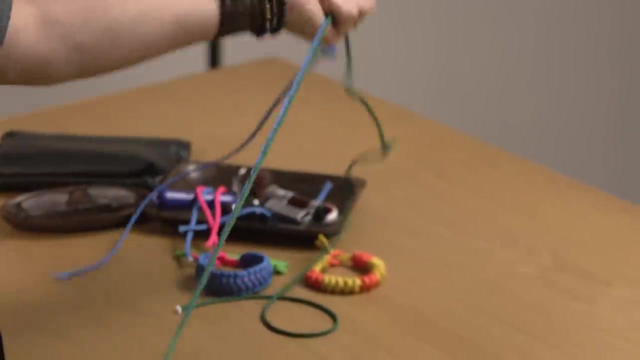 Let's hypothetically say that you made your way down from the top of that mountain, but you still have some survival needs. All you need to do is just pull out that last loop and you have all your cord ready to go and to be utilized for your next challenge. 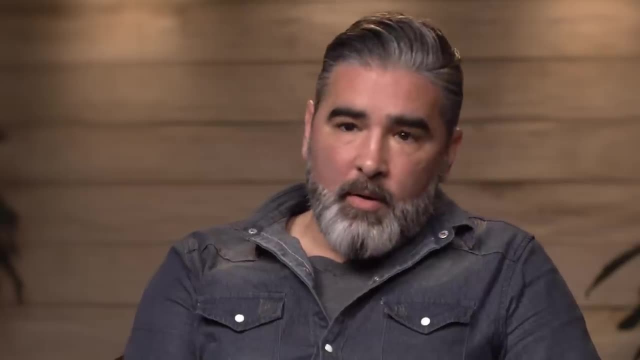 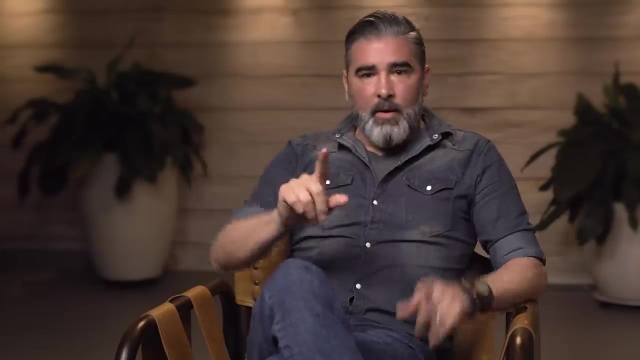 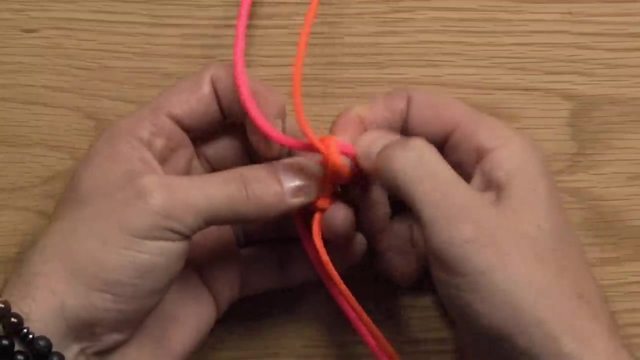 Level 13, the backbone bar. So the backbone bar it's a counterclockwise looped slip knot and a clockwise looped slip knot that is sliding onto central strands. This slip knot is going to be the place that you tuck both of those ends of cord through. 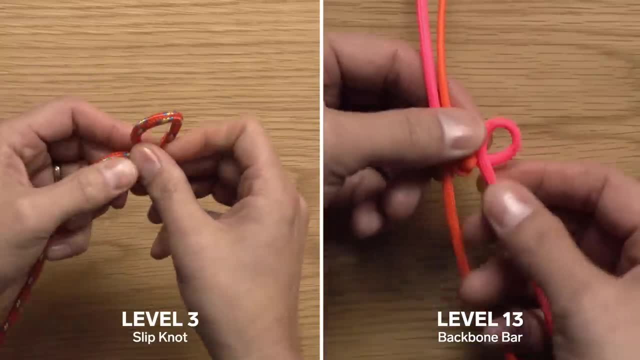 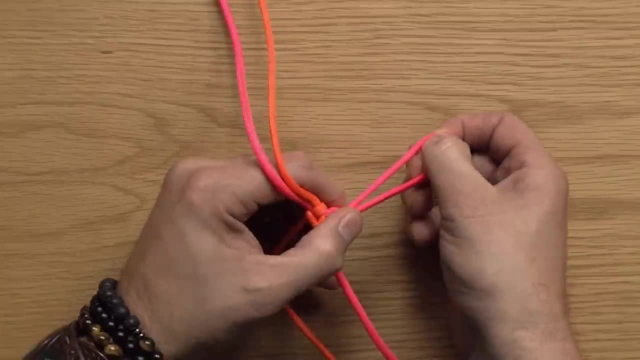 I'm going to flip it over Now. remember how, last time, I did the slip knot so that the running end was on top. This time, I'm going to do the same thing with the running end on the bottom And I'm going to slide that loop through. 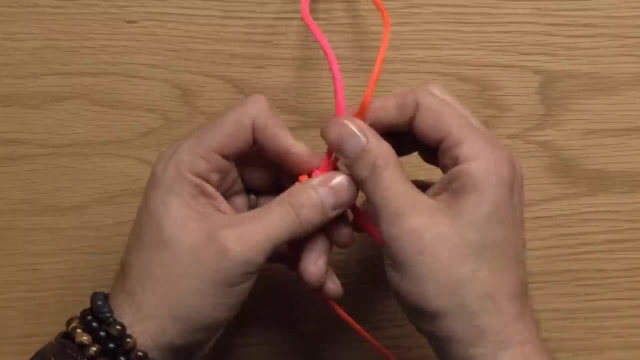 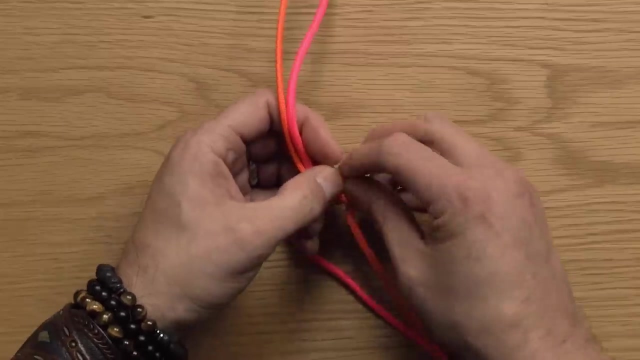 You're going to tuck both of those lines through the loop, Then you're going to turn it over and you're going to do this one on top. This is kind of a cool technique, not only just for its usefulness, because this is the most basic form of a backbone bar. 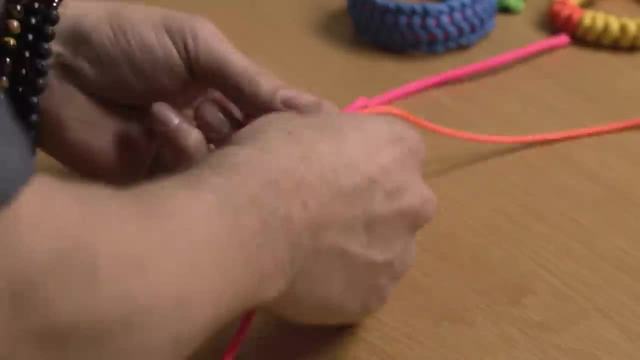 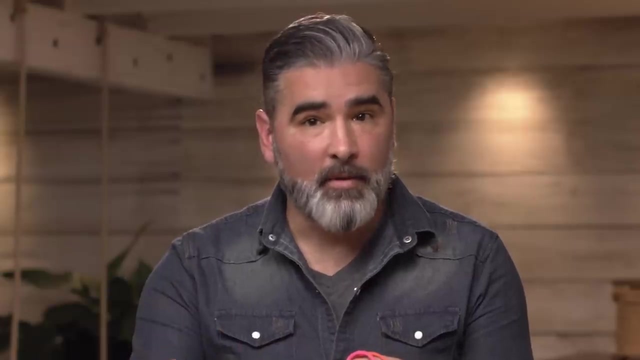 The backbone bar is- no pun intended- the backbone of other types of ties. Now that we understand the fundamental principle of the backbone bar, I'd like to show you the next level: taking this technique and utilizing it in the form of a cylindrical pouch. 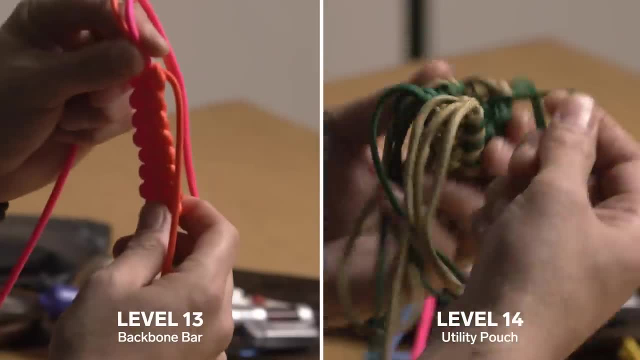 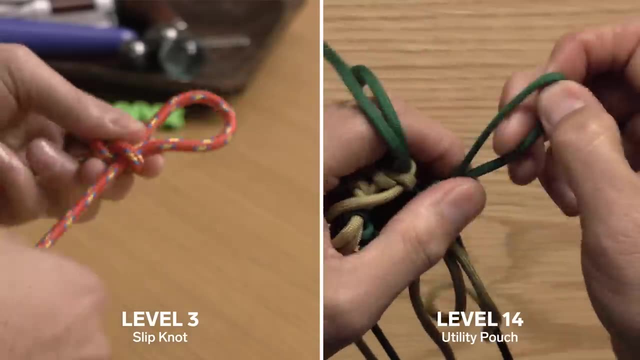 Level 14, the utility pouch. So, just as we did with the single bar, we're going to go ahead and take this line, we're going to tuck it underneath, we're going to bite that through, make a slip knot. 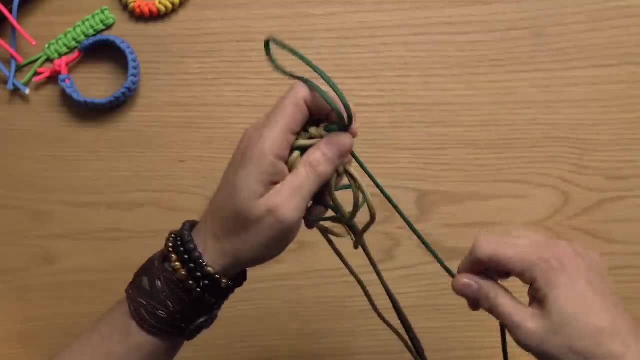 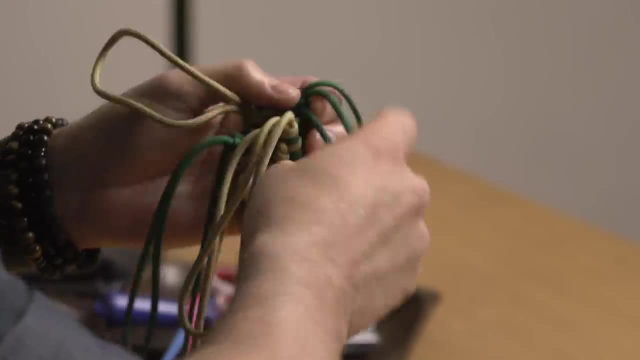 And the slip knot is going to slide over the two lines in front of it. We're going to rotate to the next position. We do the exact same thing. We're going to pull that tight. We're going to continue to do this, moving forward. 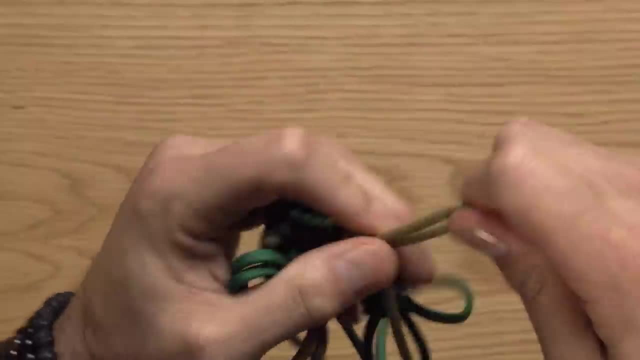 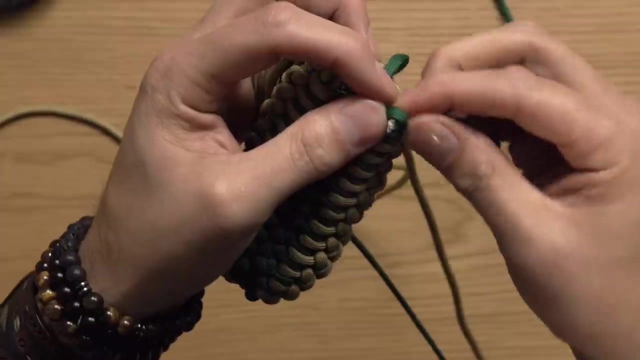 It's like a slow motion spiral made with slip knots To finish the top. all you got to do is widen that hole just a little bit fish for your end and tuck it through from the inside out. take my end. 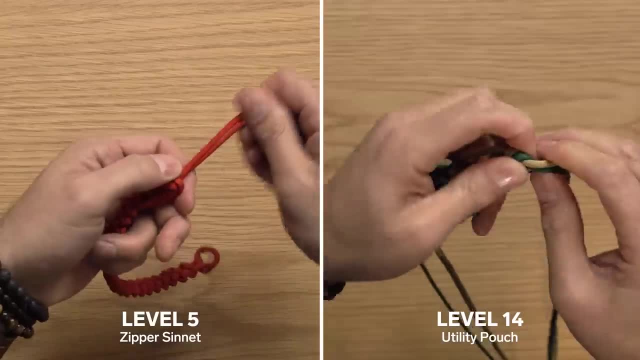 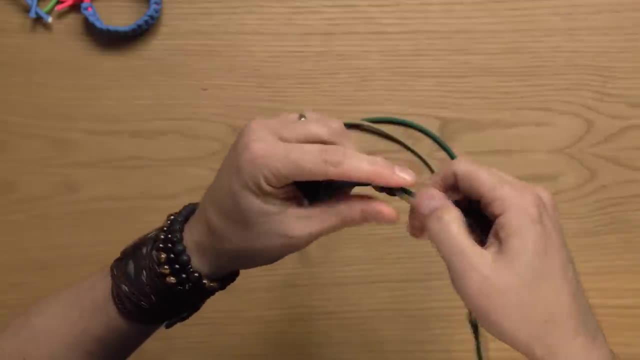 fish from the inside to the out. I'm just going to do an overhand knot, a double overhand knot. Turn it around. We're going to do the exact same thing. Once you've generated that, you don't need all this extra cord. 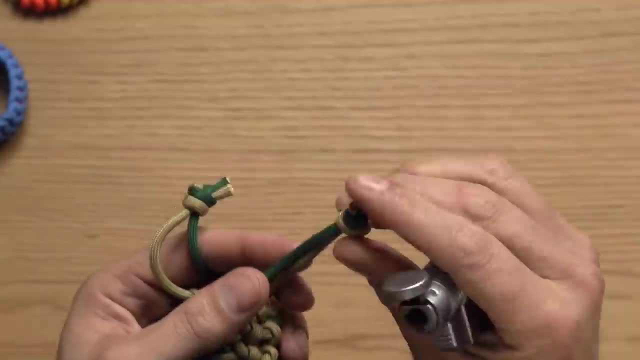 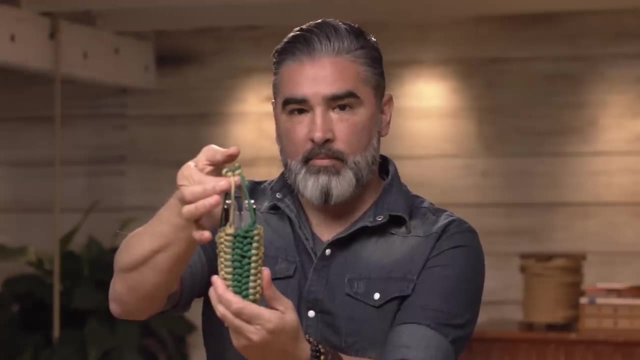 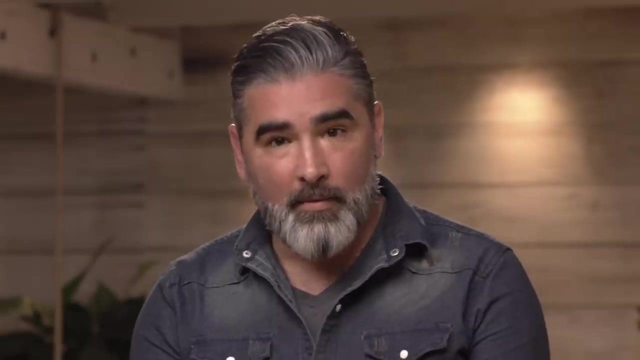 Take a little torch lighter Utility. This goes in your pouch and then this goes around the belt. Level 15, bush sandals. So the bush sandal is an elegant combination of a lot of the different elements I've already shown you today. 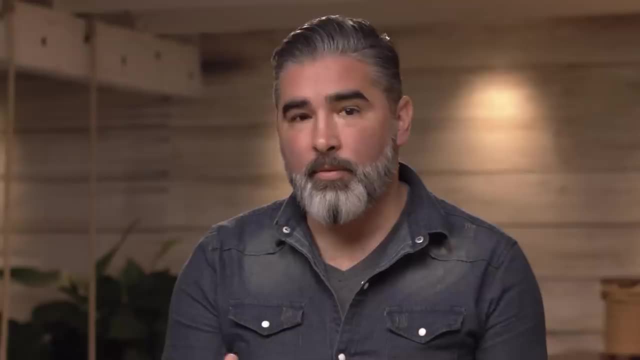 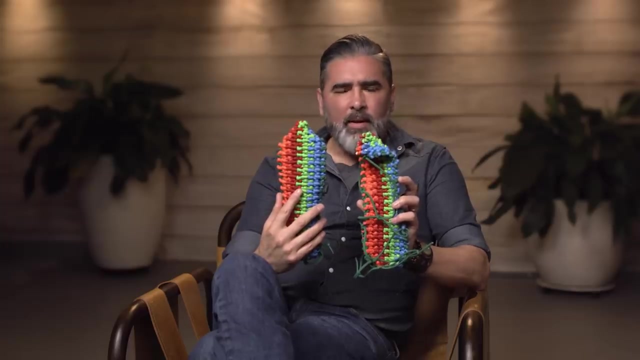 We're going to show a full hitch overhand knots and we're going to have one of my favorite knots, the slip knot, For each sandal. it takes about an hour and a half. with a little bit of leeway I would say about three. 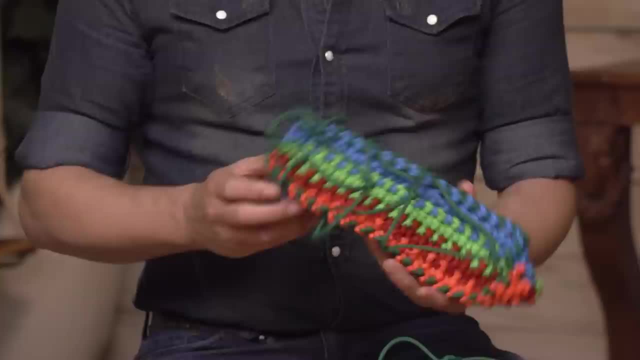 three and a half hours for both sandals. Sometimes people have come to me and said: why would I want to make bush sandals when I can buy a pair of sandals? That's a great question if you have a store nearby, But in some cases 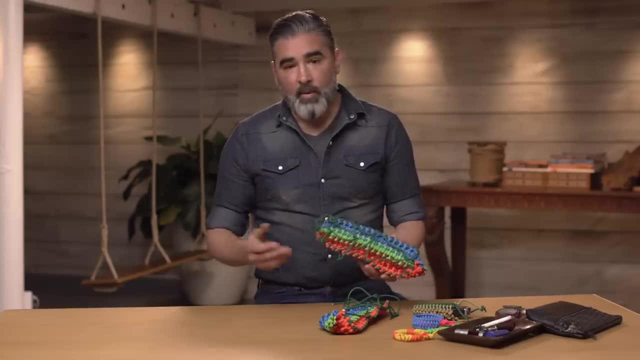 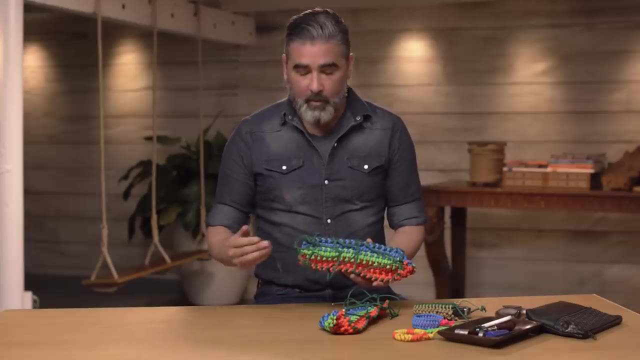 you might find yourself out in the bush and dumped, say, for example, in mud. In one instance that I personally had, I was able to pull my feet out, but I wasn't able to get my shoes out, So I found myself with socks and nothing else. 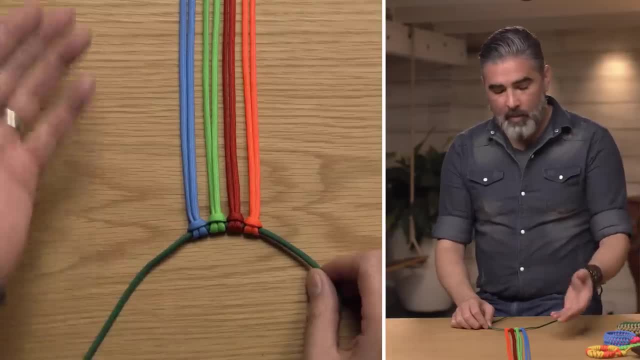 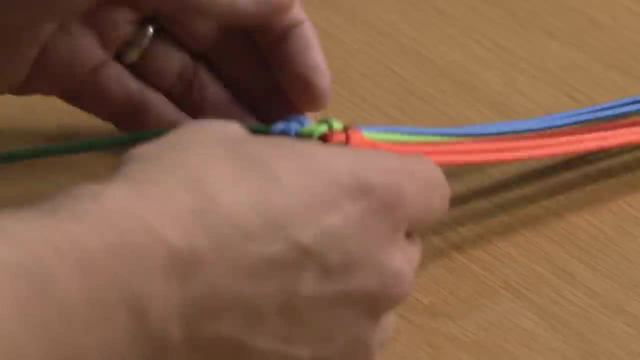 What you're going to need is five 20-foot lengths of paracord, or any cord for that matter. I made a cow hitch at the middle of the four cords. You're going to take your rightmost cord and you're going to go right over left. 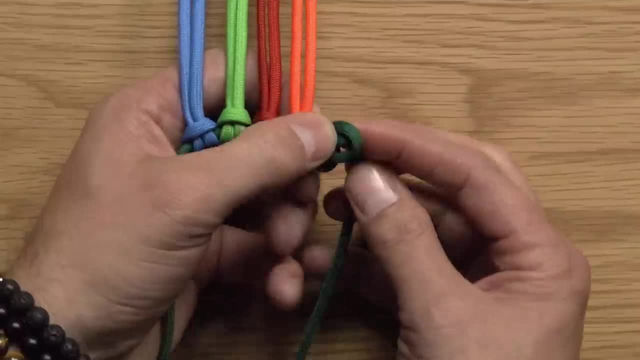 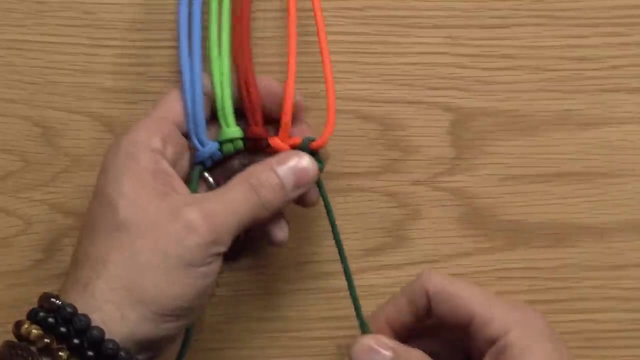 creating that familiar nine with the loop on top. Tuck through a bite, creating a slip knot. That slip knot is going to go over the cord immediately to the left. Then you're going to take the cord that you just wrapped. make your nine, punch through your bite. 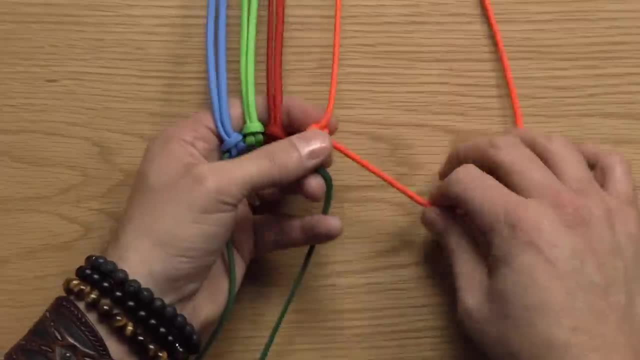 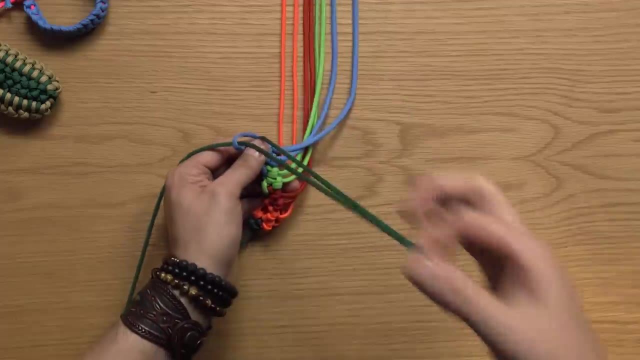 and go over the cord to its left, And then you're going to cinch that up. You might be seeing a pattern forming here. You're going to continue this all the way until you reach the leftmost side. Once you've done that, you take the entire piece. 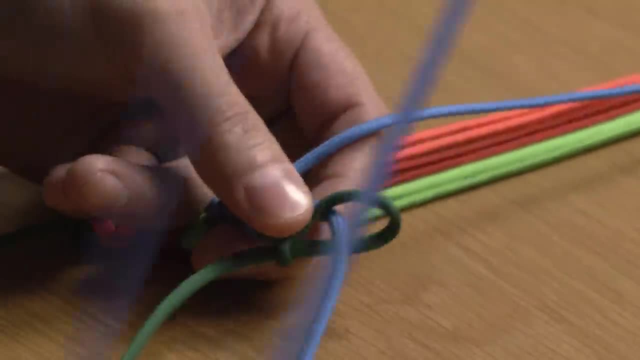 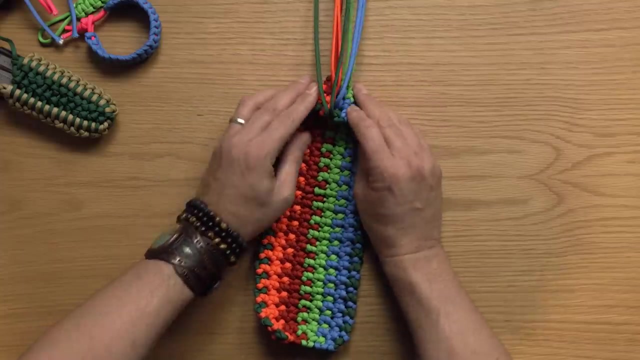 you flip it over and then you do exactly the same thing as you did before. This is what your mat's going to look like: The last knot being tied here. We're going to take this toe and we're going to compress it in. 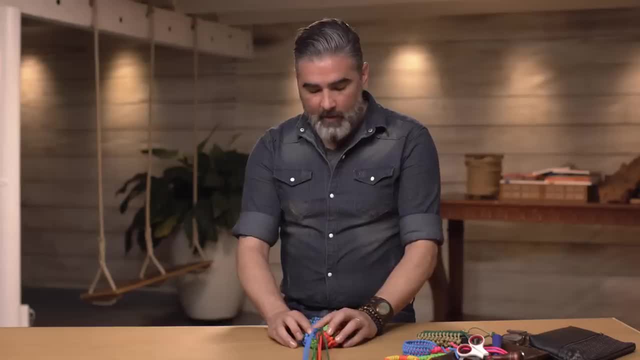 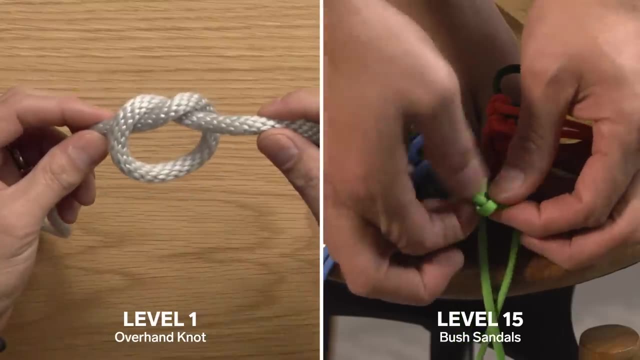 And that's going to be a protection for the front of your foot. It's also going to help kind of lock it in place in the front. You're going to take your left cord and go over your right cord to make an overhand knot. 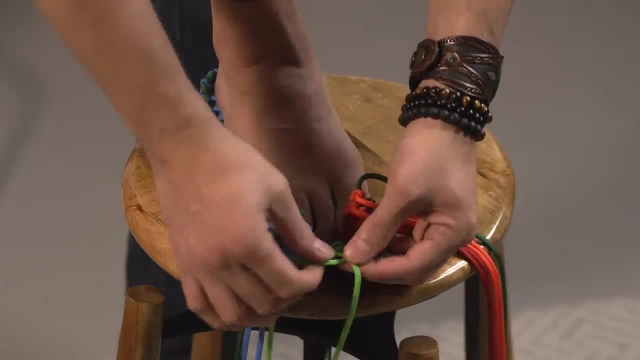 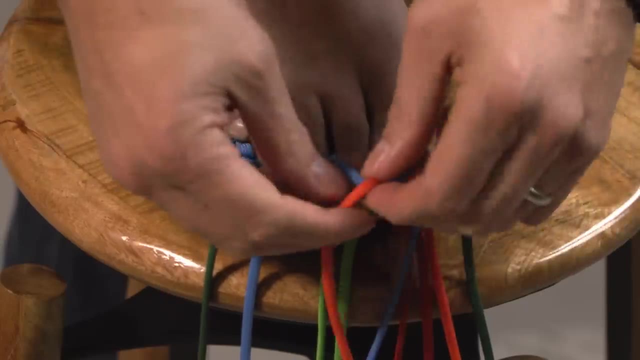 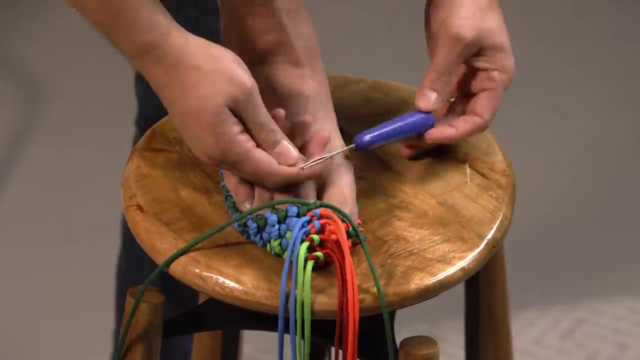 Then you're going to tuck your left cord under the right cord and over, turning your overhand knot into a square knot. Continue moving up Left over right and then left under right, And you'll notice the front of your shoe slowly curling over your toes. 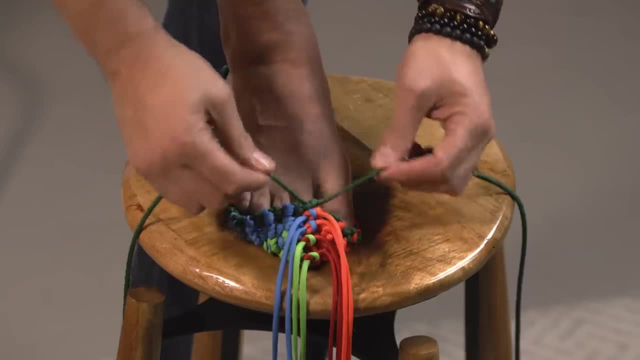 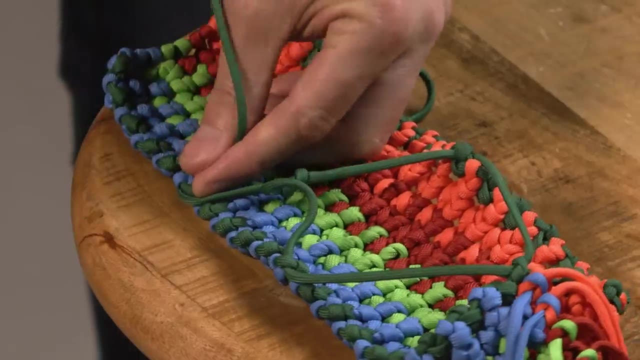 Once you've generated the last knot, you're going to measure out an equilateral triangle. Take a little tool called a splicer, Go down in between the knots just like that. This is going to come over the top, where you will tie- you guessed it- another square knot. 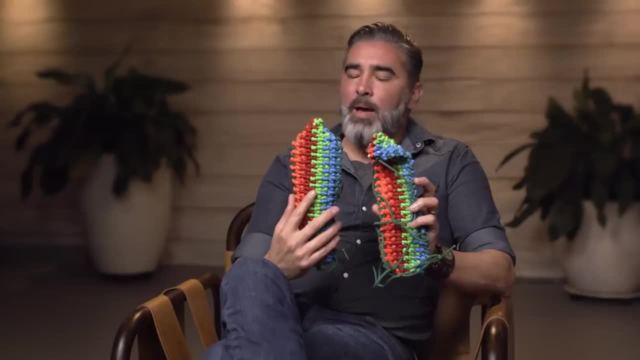 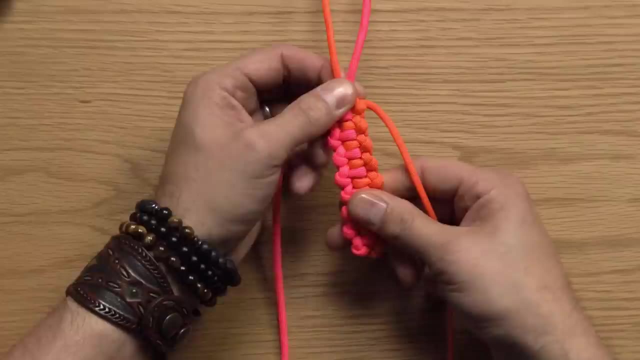 The sandals themselves feel really good on the feet, Kind of like those beaded backs that you put in cars and it triggers kind of pressure points on your feet. It feels really nice. I do not consider knotting a finite field of study.